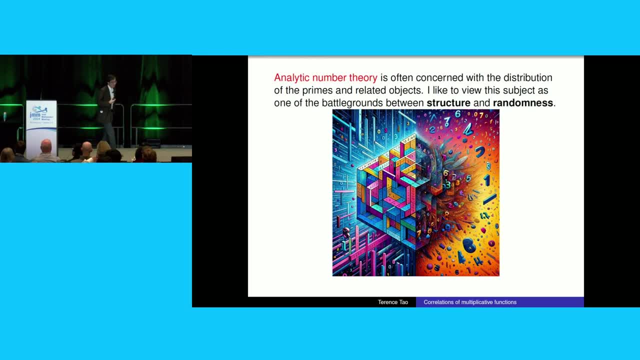 And it's because the primes are this funny object. You know they're both structured and random at the same time. You know I mean or pseudo-random, You want to be technical, since the primes are not randomly generated. You know, on the one hand, multiplicatively they behave, they have a lot of 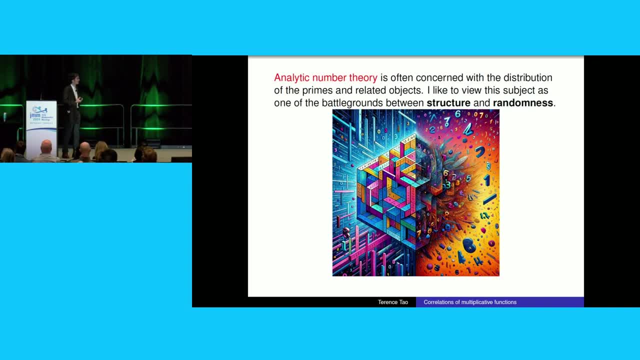 of rigid multiplicative structure, But additively they look very random, but we can't prove that in many cases. I did try to get GPT to illustrate this dichotomy with an artwork. This was its attempt. I'm not sure how successful it was in illustrating the duality of structure. 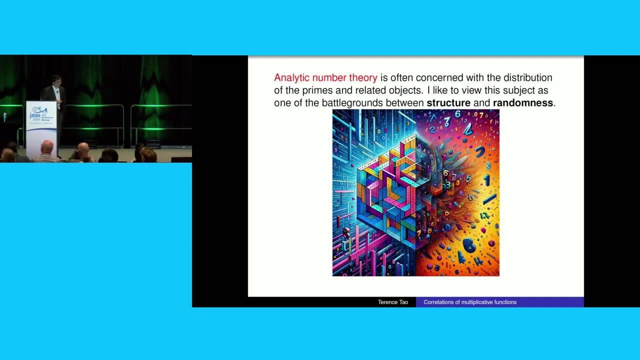 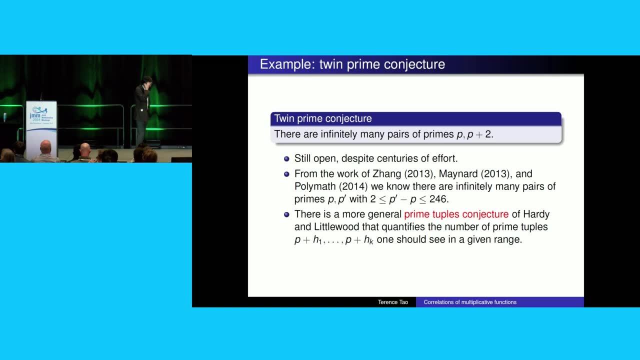 and randomness in number theory, but certainly better than anything I could do So, okay. So I mean just to give you a basic example. you know, there are many, many questions in analytic number theory that are, you know, over a century old. 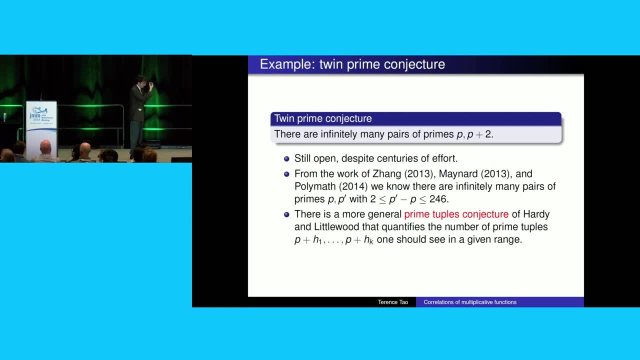 and we just have no. I mean, we've made progress but we cannot close a lot of questions. One of my favorites such is the twin prime conjecture, which goes back at least to Polignac, in like the 19th century. 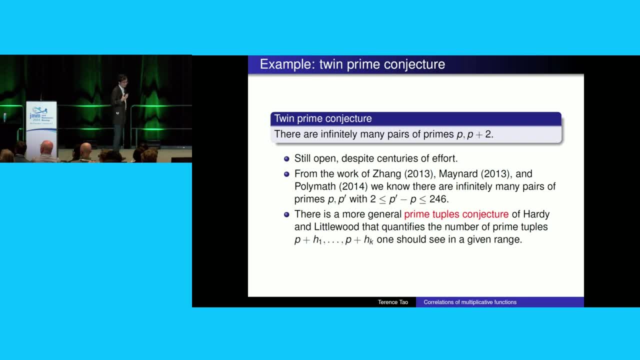 And you all know the conjecture: There's infinitely many twin primes. So we know there's infinitely many primes. Euclid did that. But we know what infinitely many primes p is is that p plus 2 is also prime, Or in other words the gap between consecutive primes. 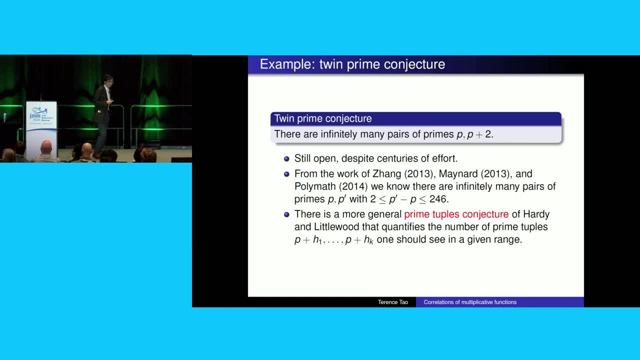 should be two, infinitely often. And that's still open. Many, many people have tried- Quite a few people have even tried to publish proofs, But it's still open. We have a lot of progress. There's a famous breakthrough of Yitang Zhang about ten years ago now. 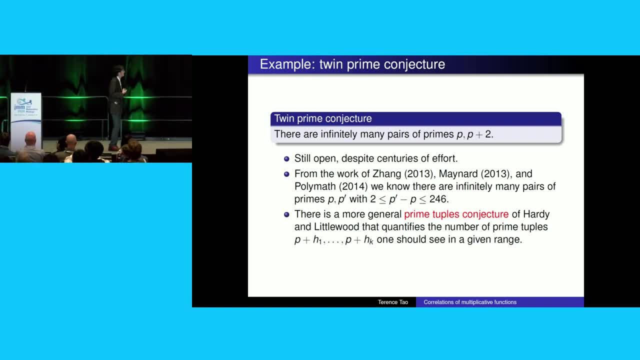 who found that there's at least infinitely many pairs of primes whose gap is at most. I think 70 million was the initial bound And it got narrowed down over well a couple of years to, and the current record is that we know that there's. 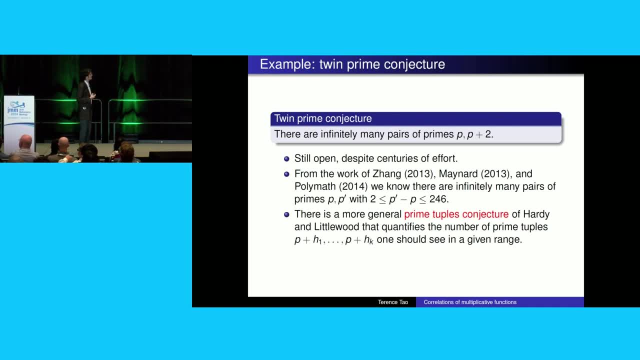 infinitely many pairs of primes whose gap is somewhere between 2 and 246.. But that 246 has stayed stuck there for about nine years, And this is just the simplest of much more general family conjectures. For example, this is a special case of something called the prime-tupos conjecture. 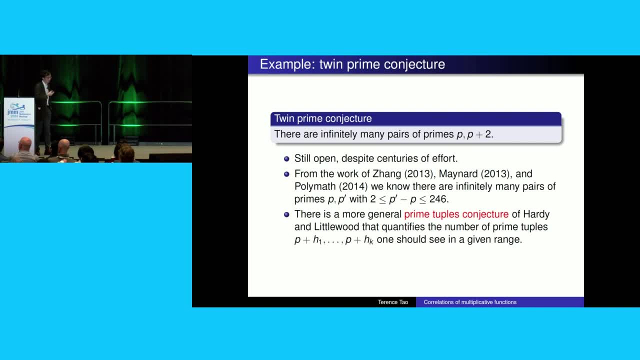 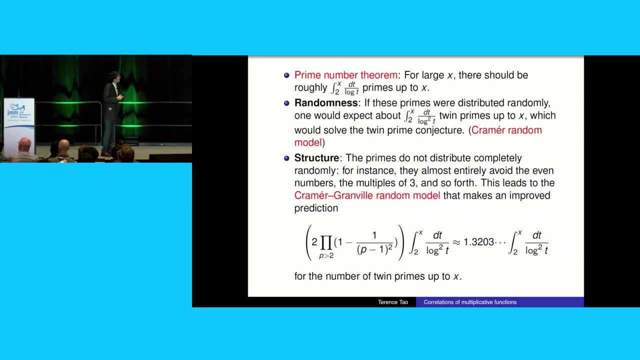 of Heiding-Littlewood, which counts not just twin primes but two pairs of primes, So it's like p, p plus 2, p plus 6, for instance. But I won't talk about this more general conjecture. 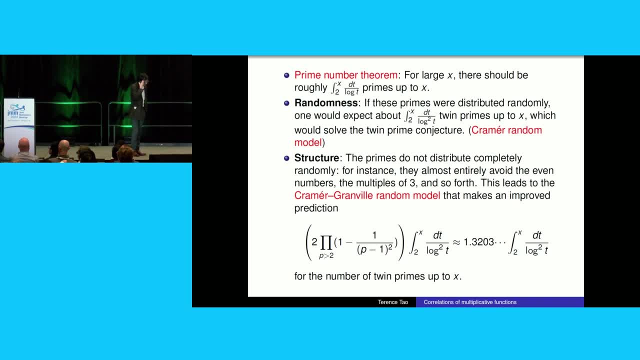 So, as I said, these are questions. So the twin-prime conjecture is true, We all know it, We just can't prove it. And not only do we know there's infinitely many twin primes, we know how many of them there are, up to some range x. 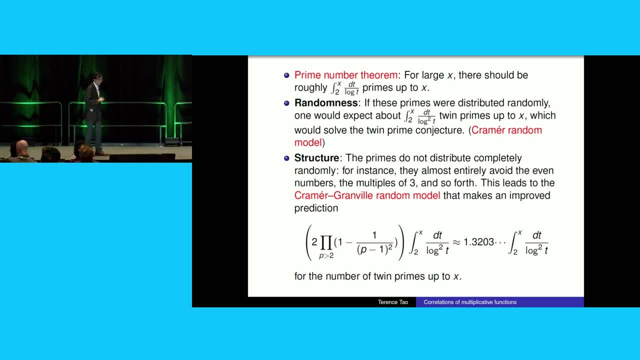 And we have all the right answers, just none of the justifications. So we have these extremely good random models of extremely reliable and accurate And so the starting point is the fundamental theorem of adding number theory, which is the prime-number theorem. We know how many primes there are, up to a large number, x roughly. 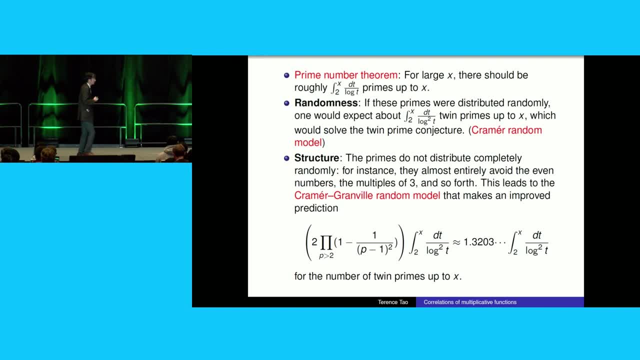 It's the log integral of x, the integral of dt over log t, from t to up to x, roughly x over log x. There's an error term which is very interesting. The Riemann hypothesis is all about exactly what that error term is. 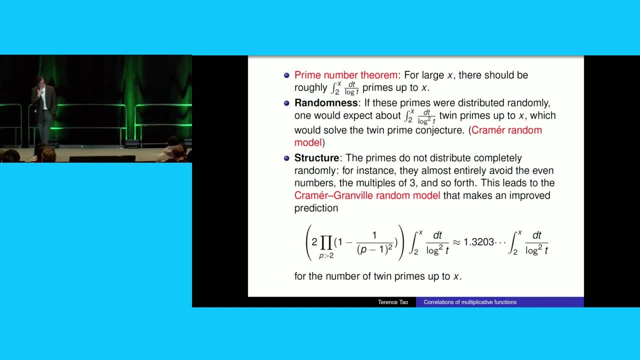 but that's not important for this talk. So we know how many primes there are in any large interval, but we don't know how they're distributed. And the first naive guess is maybe they're distributed randomly, like you take a random set of the density predicted. 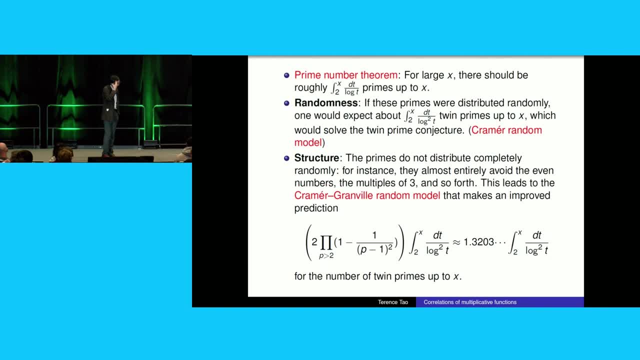 by the prime-number theorem. And if you do that, you are working with what's called the Kramer random model of the primes, a probabilistic model of the primes, and you can use that to make predictions. And if you do a naive prediction using this model, 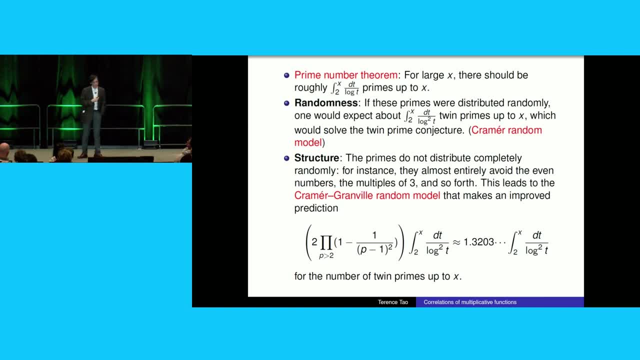 which I won't replicate here. you will predict that the number of twin primes up to x is roughly the integral of not dt over log t but dt over log squared t, which is about x over log squared x, which would solve the twin-prime conjecture. 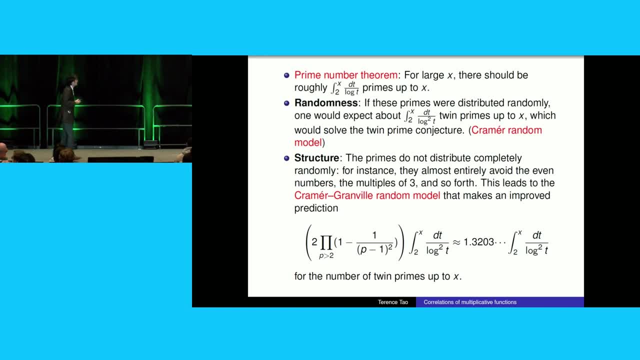 because as x goes to infinity, that goes to infinity and that would imply infinity between primes. But the primes are not completely random. For example, a random set would distribute: half its numbers would be odd and half its numbers would be even. 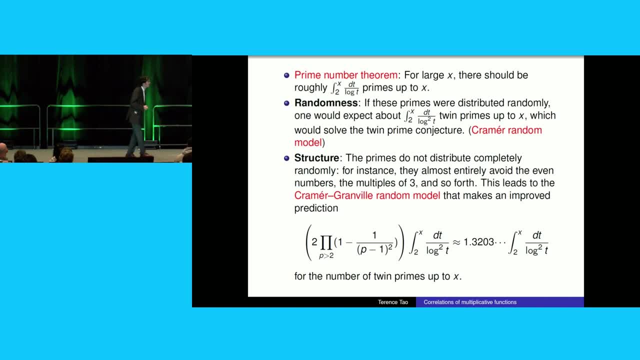 Whereas primes almost all the numbers are odd and only one of them is even So, the primes are very non-random: mod 2, and mod 3, and mod 5, and so forth. So you can modify the Kramer random model. 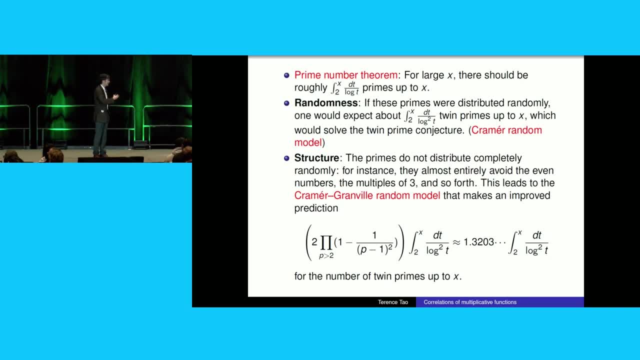 and that's what we call the Kramer-Granville random model, where you also enforce some co-primality conditions- mod small primes 2,, 3,, 5, and so forth- And this creates some adjustments to the prediction. 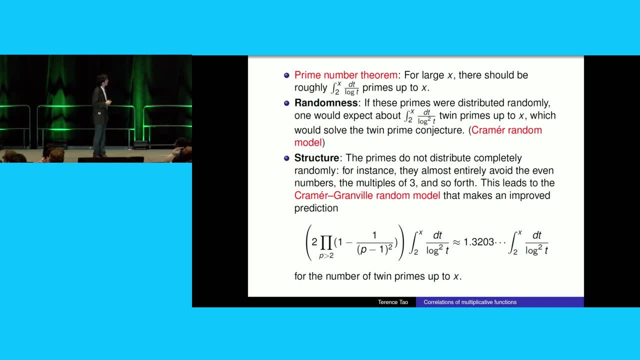 So the Kramer random model prediction is almost certainly wrong, but we can't prove that either. But we have what we believe is to be the correct prediction, which is what the Kramer-Granville random model does, And I'm not going to define this model precisely. 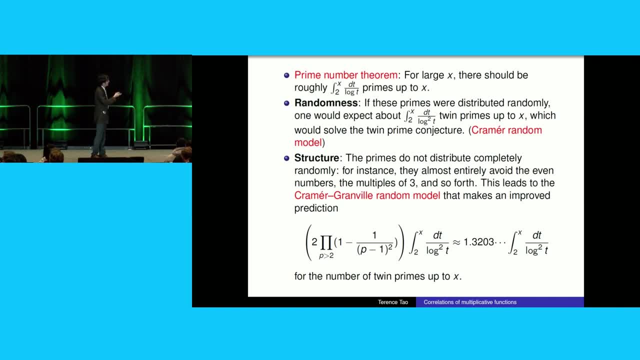 but people have, And it's the same prediction, the integral of dt over log squared t times a certain arithmetic factor called a singular series, and it's a product, 2 times a product, of odd primes of 1 minus 1 over p minus 1 squared. 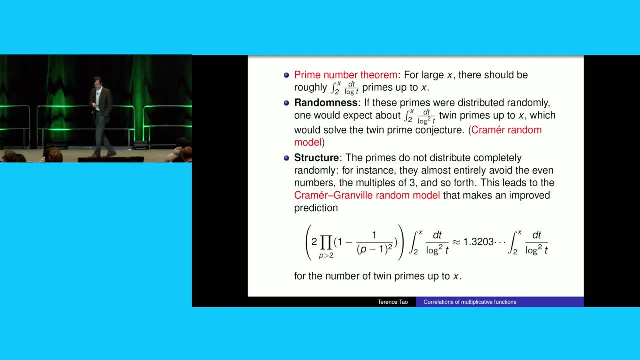 It's a specific number- 1.32 something- And so it's a corrected prediction For the number of trim primes, And so this is almost certainly true. But we can't prove this. Of course we can do numerics. 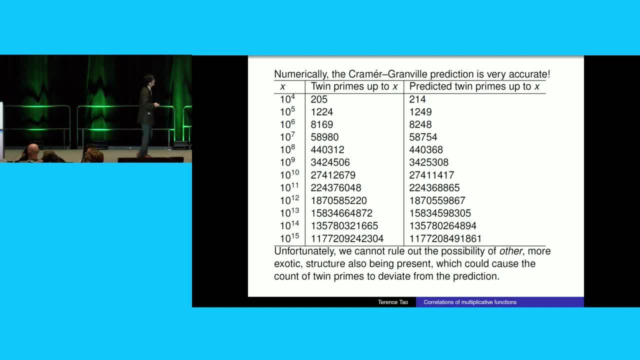 You can count how many trim primes there are, up to 10 to the 15, say and count exactly how many there are. That's on the left column And the prediction that I just wrote down. that's on the right column. 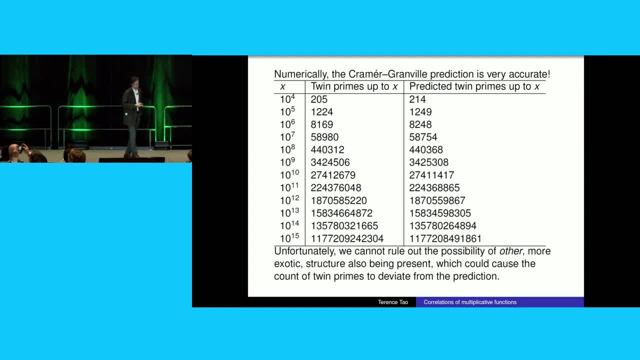 And it's accurate to, like you know at the bottom. it's accurate to what five, six decimal places, And similarly for any other kind of statistic of this type, we generally can find the right model that matches the numerics extremely well. 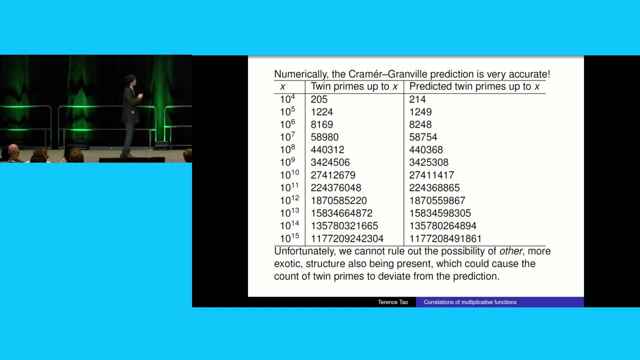 And what the accuracy of this model is kind of saying is that we have identified some obvious structure to the primes. You know that the primes avoid multiple two, multiple three, multiple five, But we don't believe there's any other special structure to the primes. 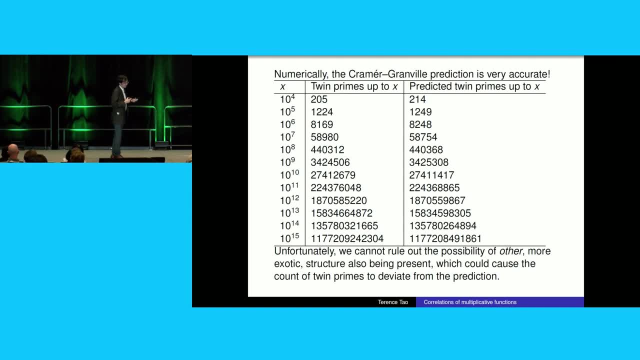 There is no tendency for twins in N plus 2 to be more likely to be simultaneously primed than not, Other than what is already coming from this local structure, There's no secret property of the primes that we've missed That we don't have to make any further adjustments. 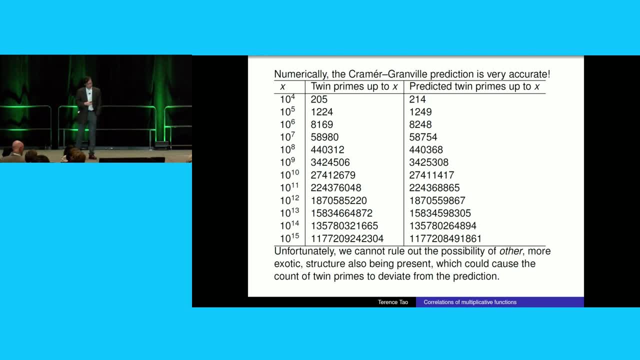 to the Kramer-Grammar model That is somehow should be our final model, But we can't do that. You know, there's always the chance that there's somehow some extra conspiracy in the primes that they have agreed to do something. 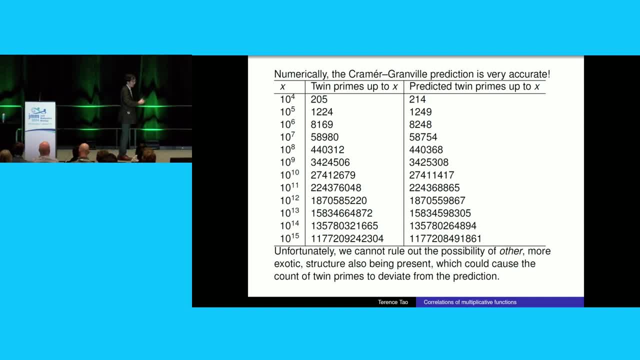 you know, if two numbers- N and N plus 2, they have some secret pact. If N is primed, then N plus 2 decides not to be primed. We don't know how to rule out these conspiracies. We can do some things with them. 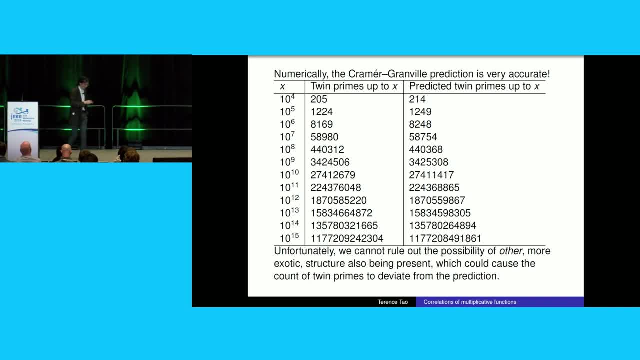 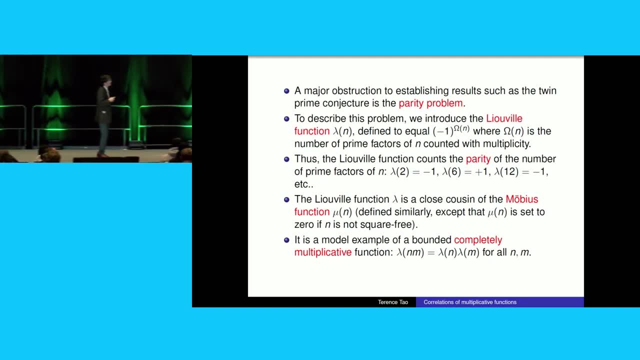 You can use one conspiracy to rule out another. That's a fun game to play, But anyway, that's not the topic here. So people have tried many, many ingenious ways to try to attack this conjecture And we still can't do it. 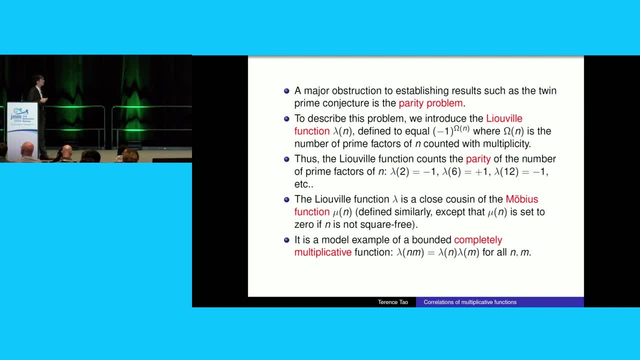 And we now have sort of an understanding why. There are multiple reasons why we can't do it. But there's one really fundamental one And it sort of shows up. It's like this big, big wall or barrier all across. I think number theory. 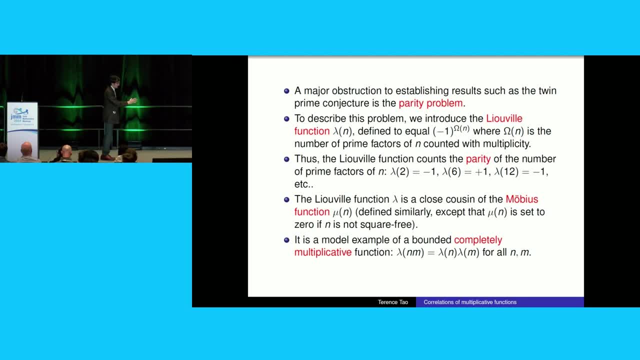 And it's stopping. you know we can all our techniques. if you're lucky you can get all the way up to this wall. Sometimes you get stuck beforehand, But it's hard to get. but only in very rare cases have we been able to breach this barrier. 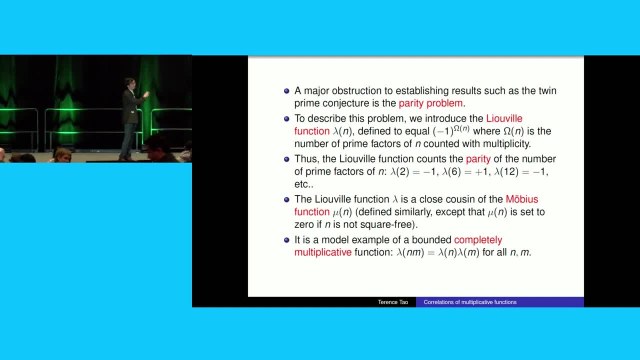 It's called the parity barrier or parity problem, And the trim prime unfortunately is on the other side of the wall. And so are many other problems that are famous and unsolved in, I think, number theory, Golbach conjecture, for instance. 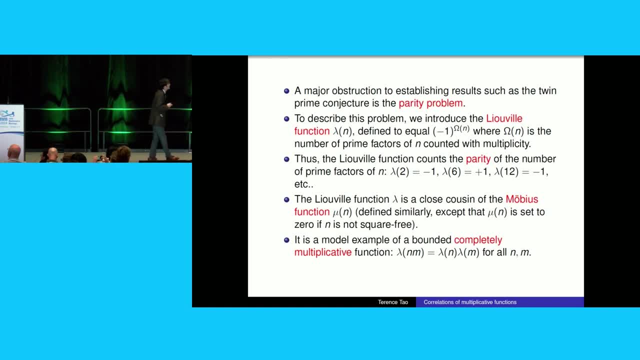 So what is the parity problem? So I need some notation, So I'll introduce what's called the Louvre function. So this is a fairly simple function. It's just it's defining the natural numbers lambda of n, And it's either plus or minus one. 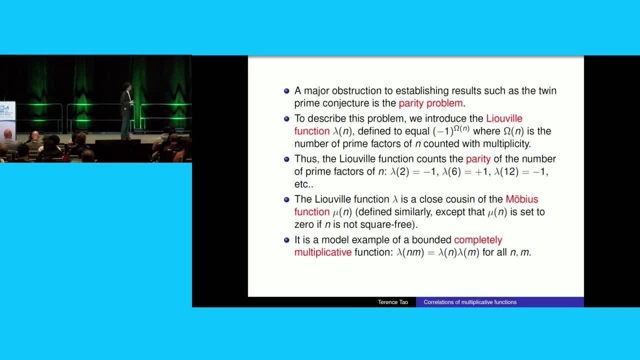 It just counts the parity of prime factors. So if you're the product of an even number of primes, it's one, And your product of an odd number of primes is minus one. So it doesn't exactly count whether you're prime or not. 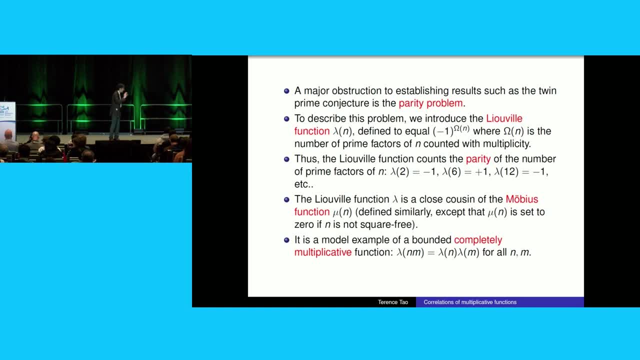 It just counts whether you have an odd or even number of primes. It just counts the parity of primes. And if you have multiplicity, if a prime appears multiple times, you have to count it with multiplicity. So, for example, lambda of four would be plus one. 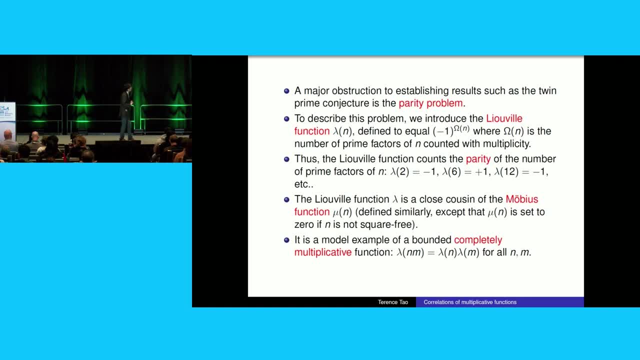 because four is two times two, You have an even number of primes in your factorization. Okay, so just some simple examples there, Lambda two is minus one, Lambda six is plus one. It's a simple function. There's a more famous cousin of the Louvre function. 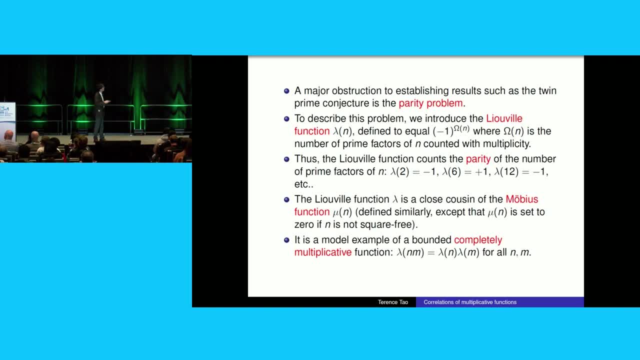 called the Mobius function, which is almost the same function, except that the Mobius function is supposed to vanish if you are not square-free, But the Louvre function we define to still be plus or minus one, even if you have repeated prime factors. 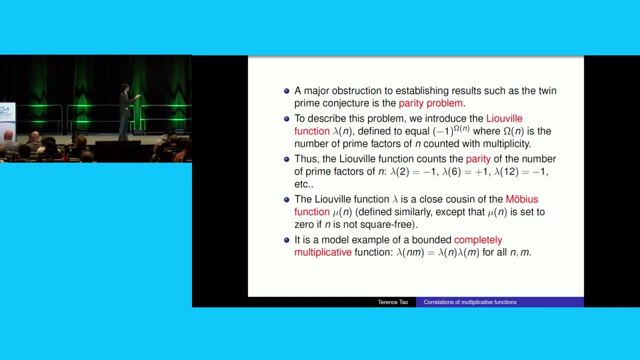 But they're pretty much, They're almost identical. Pretty much everything we know about the Mobius, we know about Louvre, and vice versa. Louvre is just a tiny bit more convenient for me to talk about today, so I'll try to focus on Louvre. 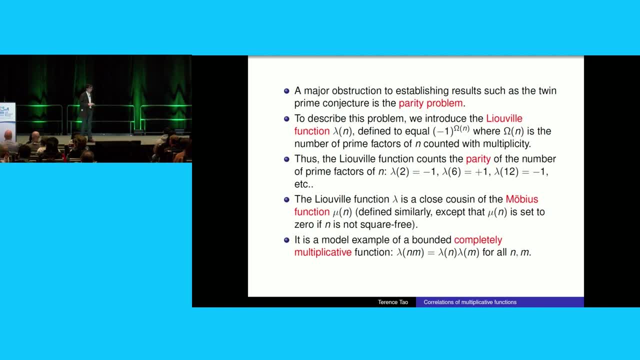 For example, Louvre function has a nice property. Well, first of all it's bounded. It's always plus or minus one. It doesn't go to infinity. But it's also what's called completely multiplicative, If you take lambda of n times m. 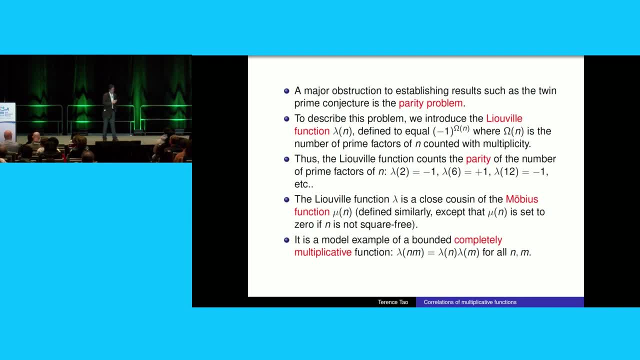 it always factors into lambda of n, times lambda of m, If you like. it's a homomorphism or a character. Mobius function is almost, It's just called, multiplicative. The same identity only holds if you end up at co-prime. 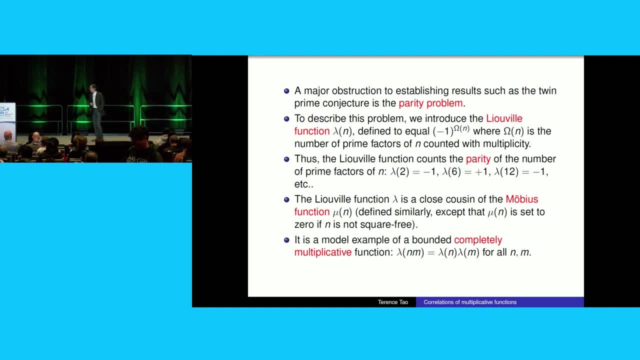 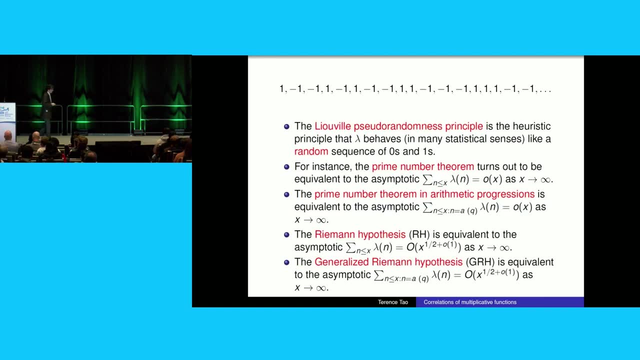 So it's just slightly less convenient. So that's one reason why I want to work with the Louvre function. Okay, so it's a function that counts parity, And if you just So, here are the first. I think 15 or so. 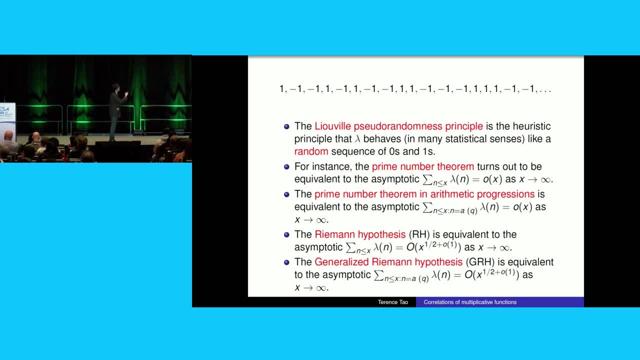 So lambda of 1 is 1.. Lambda of 2 is minus 1.. Lambda of 3 is minus 1.. And it just If you look at the, If you stare at long strings of the Louvre function, it just looks like a random string of plus or minus 1s. 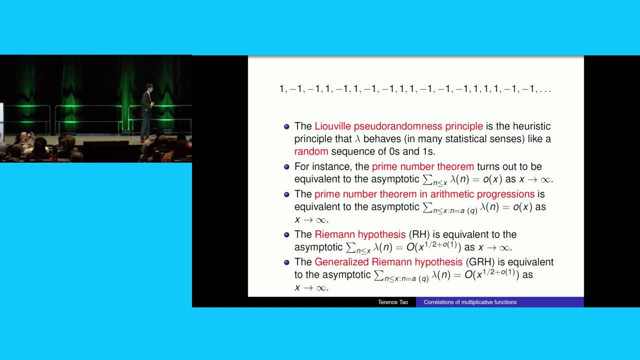 And you know you can actually subject the sequence to various statistical tests to try to see if you can distinguish it from a sequence of random plus or minus 1s. And in many statistical tests it just looks indistinguishable from random sequences. 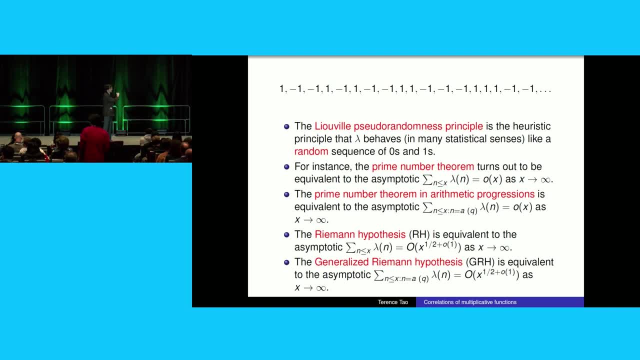 Of course it's not random. There's only one Louvre sequence And we just saw it's completely multiplicative. So when viewed multiplicatively, there's a huge amount of structure. This function is very structured multiplicatively, But additively, if you look at, say, consecutive elements. 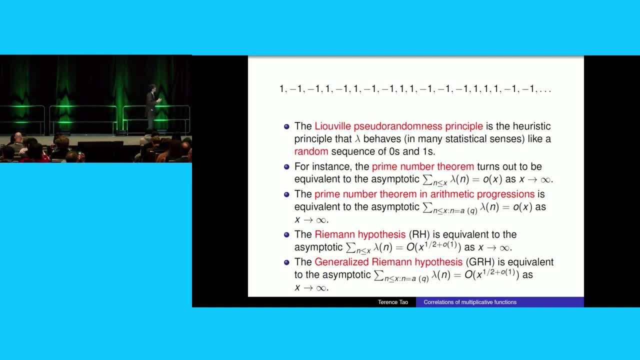 or a block of 10 consecutive elements, the Louvre function. it's very hard to distinguish this from a block of 10 random plus or minus 1s, And in fact there's a general principle in number theory, analytic number theory, called. 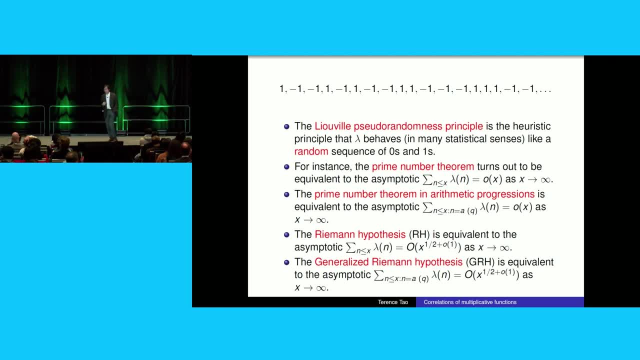 Well, it's often called the Mobius pseudo-randomness principle, But in this context it would be the Louvre pseudo-randomness principle, which basically tries to say that this is what you'd expect. So outside of sort of the, As long as you're not dealing with a purely multiplicative problem, 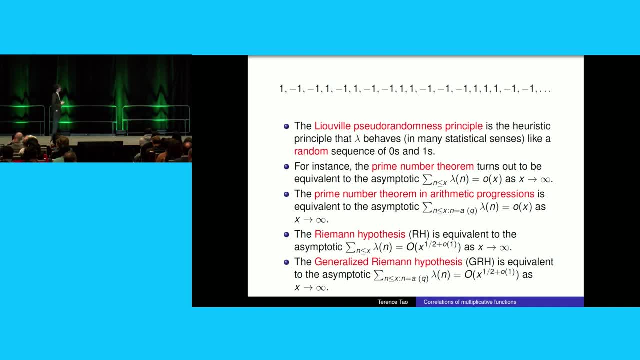 the Louvre function should statistically look like a random sequence, And this sort of supports or This can be used as heuristic justification for all kinds of both theorems and conjectures in analytic number theory, For example the prime number theorem that we mentioned previously. 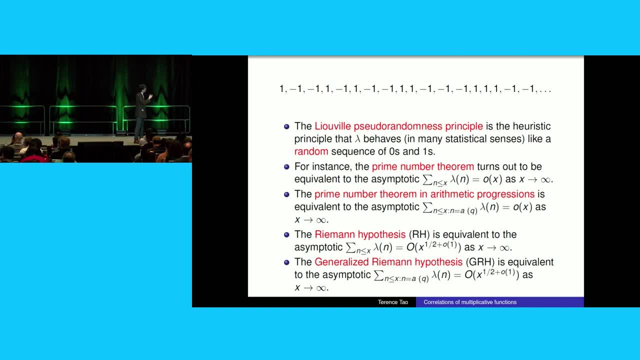 there's some very elementary manipulations. It turns out that the prime number theory is equivalent to the assertion that the Louvre function has asymptotically mean 0. That if you take the sum of the first x values of the Louvre function. 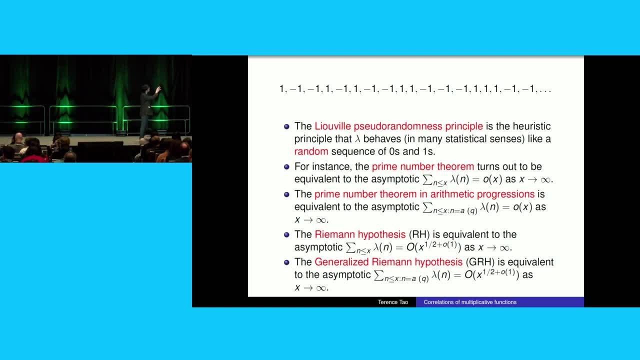 divided by x, that should go to 0. Or, if you like, about 50% of the time the Louvre function will be plus 1 and 50% minus 1. And of course, that's what random sequences do. 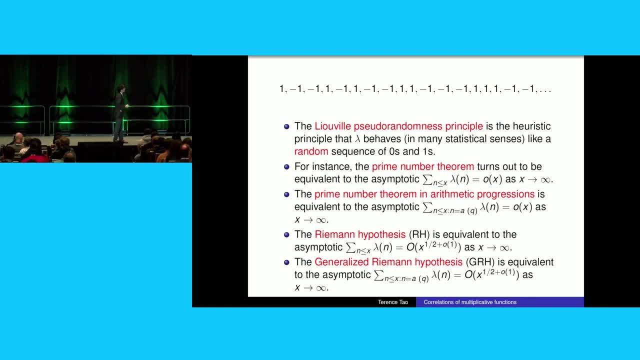 That's the law of large numbers, And so that's. I mean, that's not the only thing that random sequences do, but that's one thing that random sequences do, And so the prime number theorem is in some sense justified by this. 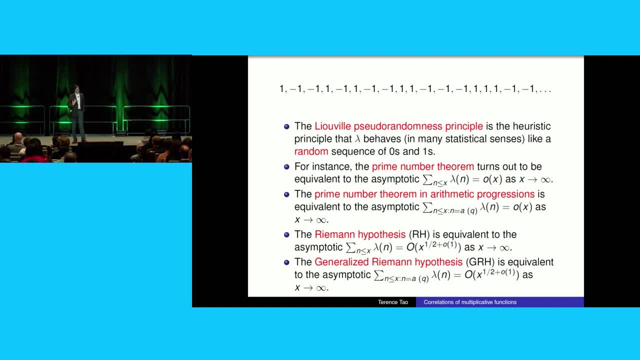 to the randomness principle. A very similar argument shows that the Louvre function should be equidistributed in any arithmetic progression. If you look at all the numbers that end in 7, mod 10, you know half of them should have even parity. 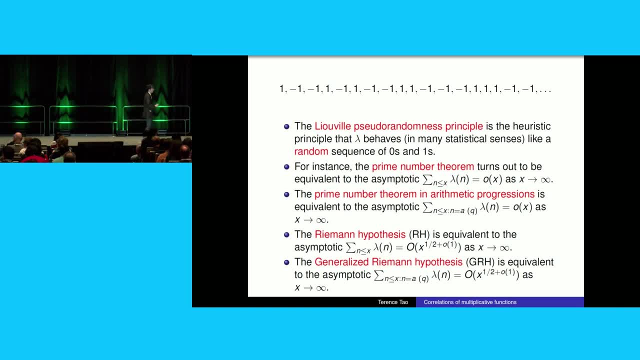 and half should have odd parity: One half the time and minus one half the time. We can prove that, And that's equivalent to what's called the prime number theorem in arithmetic progressions. The Riemann hypothesis also can be phrased: 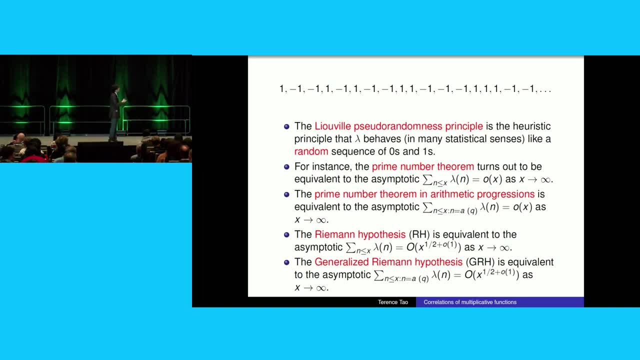 in terms of the Louvre function. The Riemann hypothesis actually is equivalent to the assertion that if you take the sum of the first x values of the Louvre function, it should not only decay faster than x, it should actually decay like square root of x. 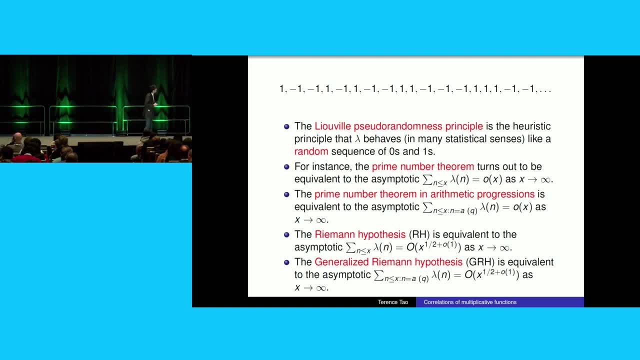 up to a log factor which I won't talk about, which is very interesting. There's another story, But that is Yeah, which, And that's what random sequences do That's more likely to do with the central limit theorem and the law of the double iterated logarithm. 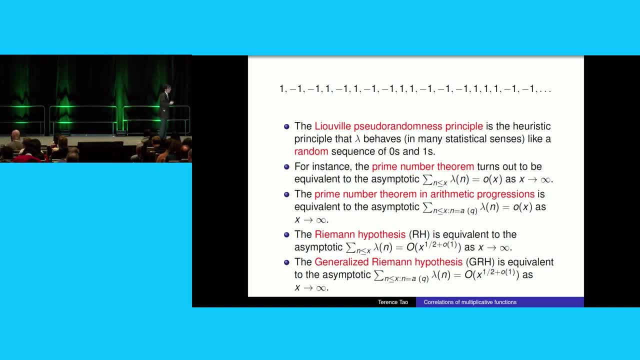 But again, the probabilistic heuristics support the Riemann hypothesis, something called the generalized Riemann hypothesis, which is sort of the same thing in arithmetic progressions, roughly speaking. Okay, All right, So let's make some more notation. 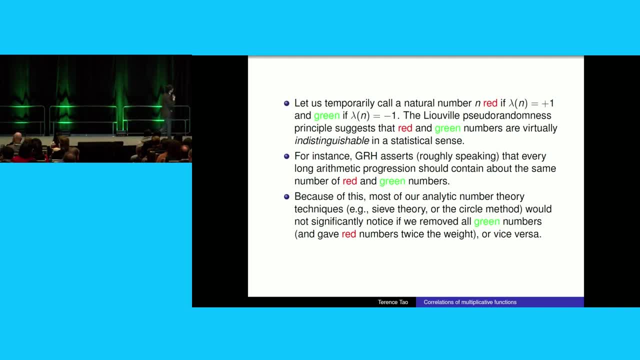 So you can think of the Louvre function as if you're a commentator on this. you can think of it as a two-coloring of the natural numbers. So let's arbitrarily call a natural number red if the Louvre function is plus one. 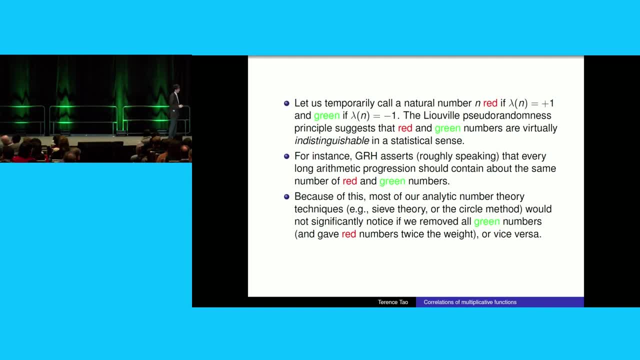 so it's a product of even number of primes and green if it is minus one. So you know half the numbers are red and half the numbers are green And the Louvre function is plus one, so the Louvre pseudo-randomness principle. 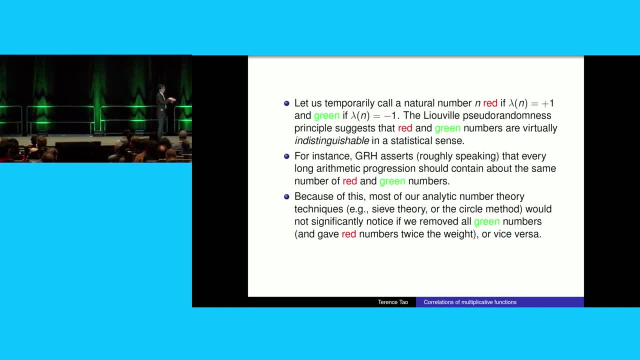 suggests that somehow the red and green numbers are just statistically indistinguishable. You take any statistical test for the red numbers and the green numbers, you can't tell them apart. And also correlations, you know like. if I won't precisely say what I mean by that. 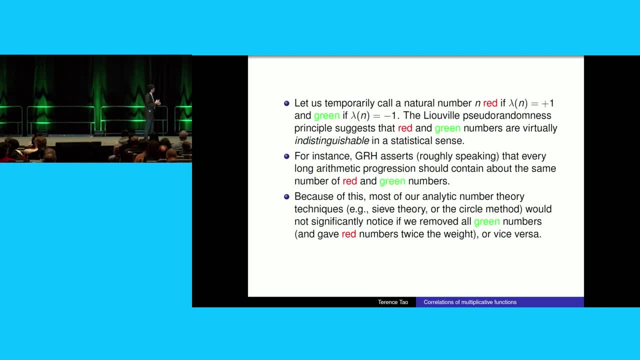 Okay, I'll just say that GRH, for example the generalized Riemann hypothesis, roughly says that every long ethnic progression should contain about half- you know should be half red and half green And pretty much any other interesting set which isn't just a set of red numbers. 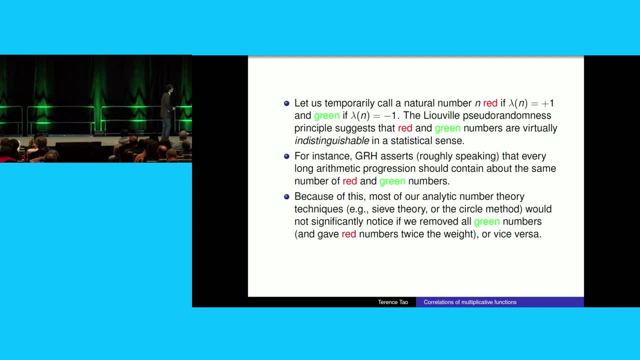 or a set of green numbers should contain 50% red, 50% green. So Okay, so this is sort of a heuristic. One consequence of this is that if you somehow decided to delete all the green numbers in the world and keep the red numbers, but make them twice as heavy, 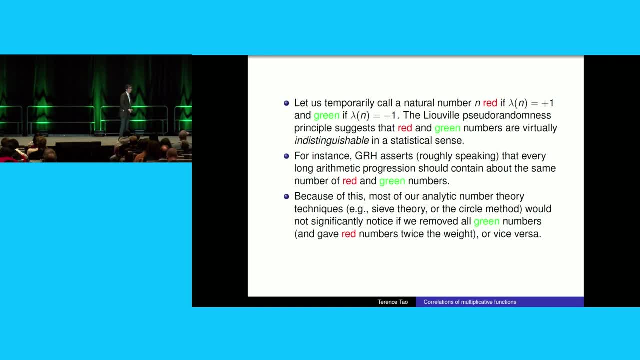 so you give the red numbers a weight of two and the green numbers a weight of zero. that should statistically be indistinguishable, as if you both have the red and green numbers with a weight of one, or if the red numbers have a weight of zero. 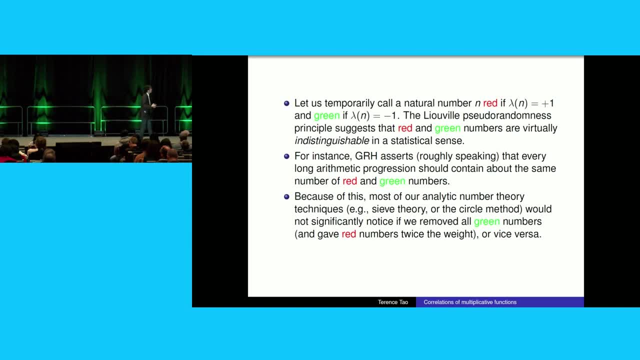 and the green numbers have a weight of two, So there are different weights. you can put on the natural numbers And And like if you count how many of What's the weight of an ethnic progression, it should be the same. 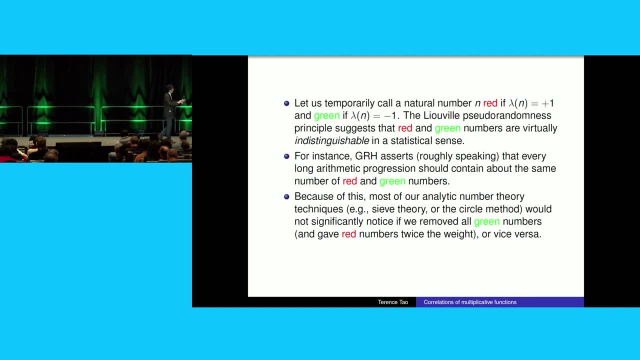 All three weights would be indistinguishable. There are many, many statistical tests for which you cannot tell the difference between these measures And many of our techniques in adding number theory, kind of a sieve theory or the circle method, just to name some examples. 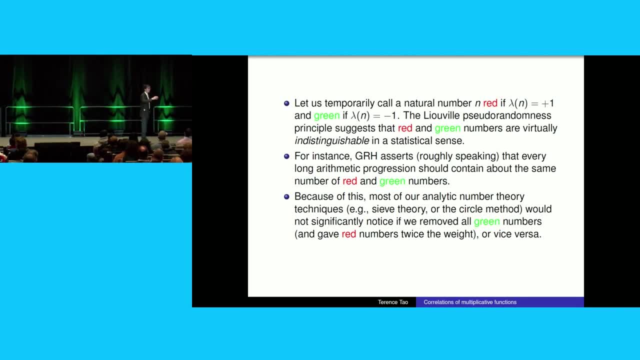 they're kind of colorblind. They can't tell If you secretly replace the uniform measure on the natural numbers with the one in which you remove the red numbers and make the green ones twice as heavy, or vice versa. they can't tell, Like all the base inputs of sieve theory. 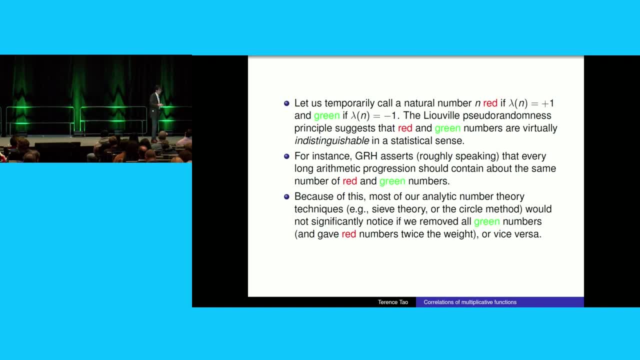 or the circle method, they. This is a blip in the arrow terms. Nothing really changes, And so any result that you can prove using standard ethnic number theory techniques, with a few exceptions. There are some key exceptions which are color-sensitive. 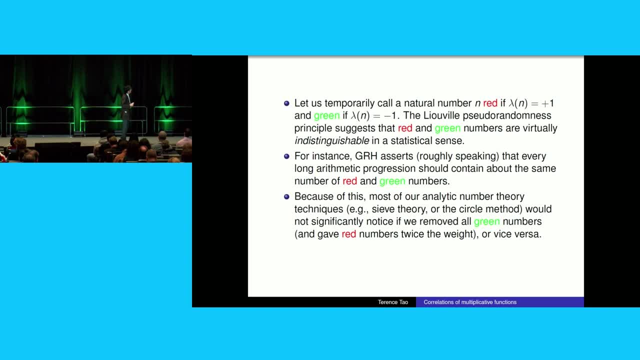 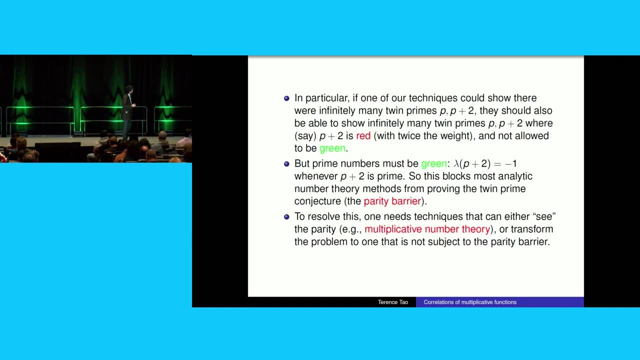 but parity-sensitive. But many of our techniques are parity-insensitive and they won't notice if you've changed the measure on your natural numbers in this way. And that's a problem for things like twin primes, because you know if you want to count twin primes. 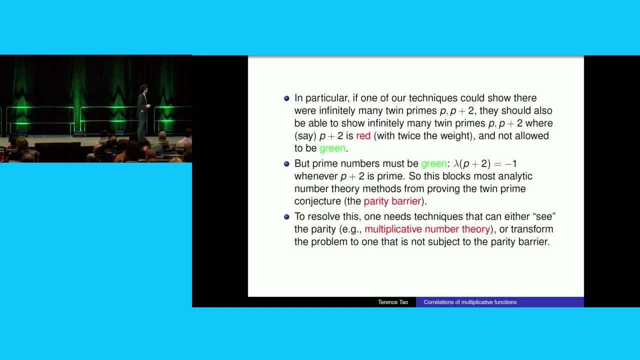 and you decide to re-weight the natural numbers based on, say, the color of P plus 2, so if you arbitrarily decide to make red numbers P plus 2 twice as heavy, the red numbers end with N plus 2, red twice as heavy. 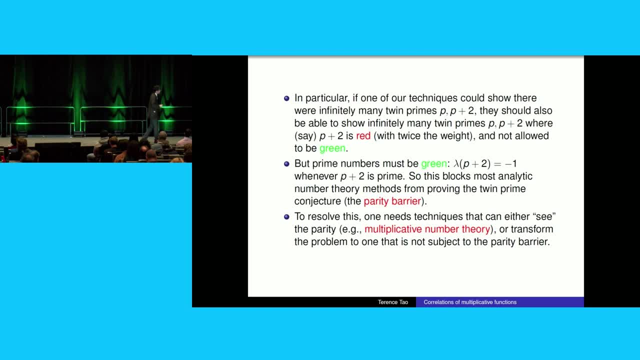 and the red numbers end with N plus 2 green, you delete them. a lot of our techniques in sieve theory would not notice and a lot of techniques in the circle method would not notice. And so whatever predictions these methods can give or whatever rigorous results they can give, 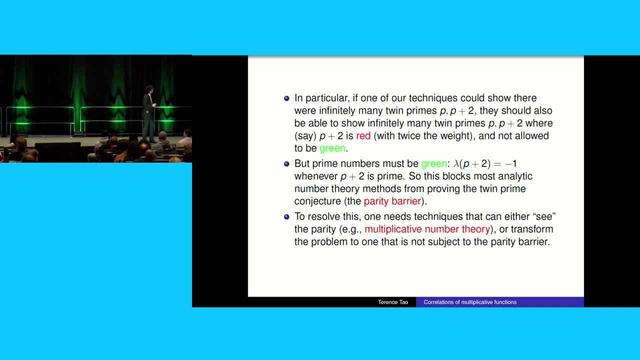 for the standard weight, they can give for this other weight as well. But if you do that kind of weighting, for example, if you delete all the green numbers, N where N plus 2 is red is green and you only keep one, you have red. 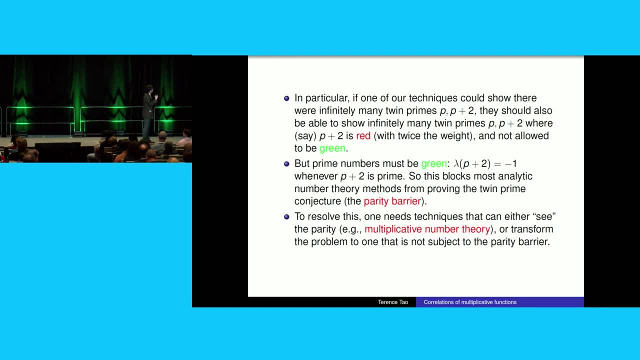 you have deleted all the twin primes, because the Louisville function is minus one at the prime Primes are always green. So if you've deleted the numbers where N plus 2 is green, you have deleted- yeah, twin primes in particular. 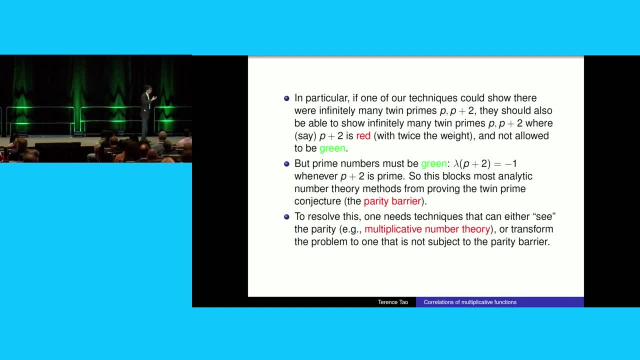 Yeah, so this was a very vaguely stated argument, but there's a nice formalization of this by Selberg, Yeah, And Bombieri and a couple. there are ways to make this argument really quite precise, And so this blocks a lot of any number theory methods. 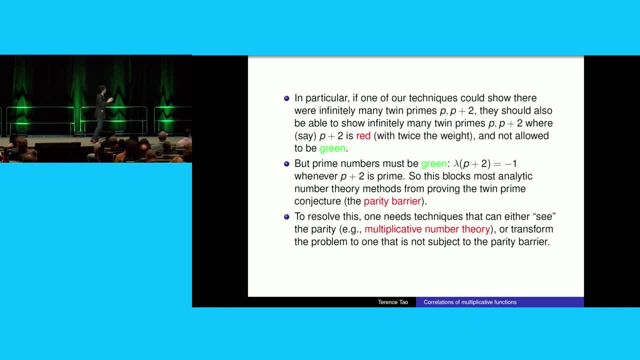 from proving things like the twin prime conjecture. There are a few techniques- and they're very precious to us- that can somehow ask parity sensitive. So the biggest one is multiplicative number theory. I mean, if you actually use the multiplicative property. 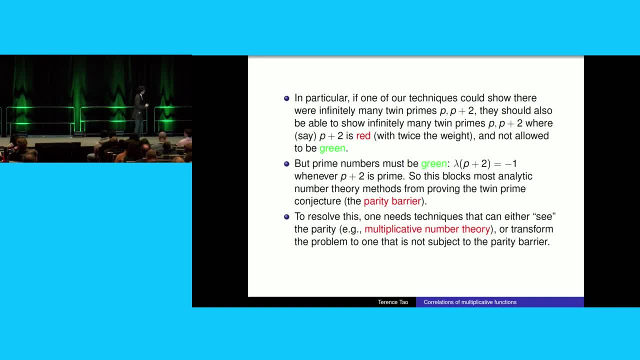 like red times red equals red and red times green equals green and so forth, then you are actually being parity sensitive. So we can prove the prime number theory, for example, but using multiplicative number theory methods, like using the Riemann zeta function. 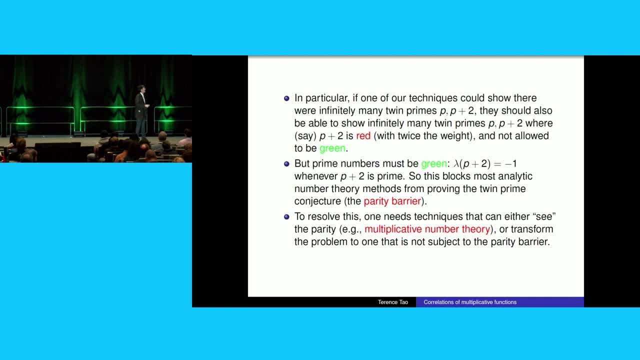 but we cannot prove the prime number theory with just some sieve theory. Well, okay, you can with a lot of extra effort, but that's another story. Okay, There's a lot of extra stories that I really cannot talk about. Okay, but all right. 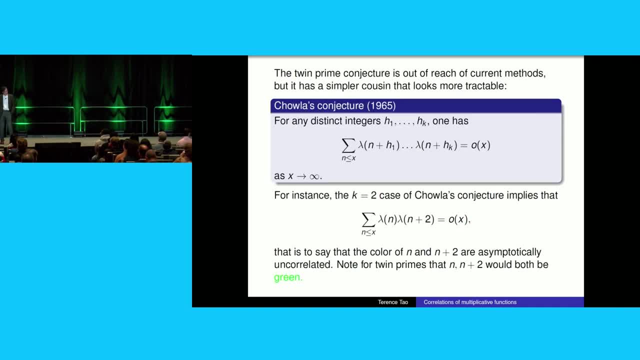 All right, Okay, so the twin prime conjecture is too hard, But it has a cousin which is easier. So one of the reasons is so the parity barrier is one reason why it's hard. Another problem is that primes are sparse. 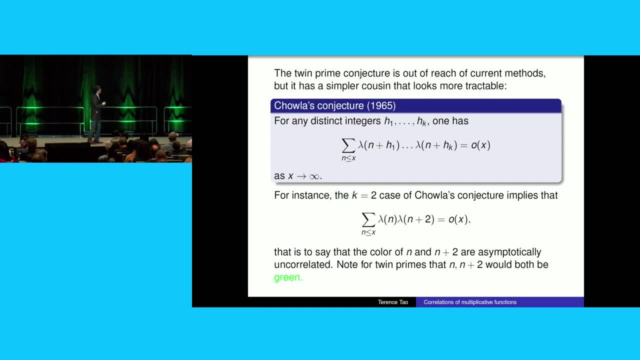 They have asymptotically density zero And that creates a whole bunch of separate problems, which, again, great story. I can't talk about it today, But you can work with non-sparse, you can work with a non-sparse version. 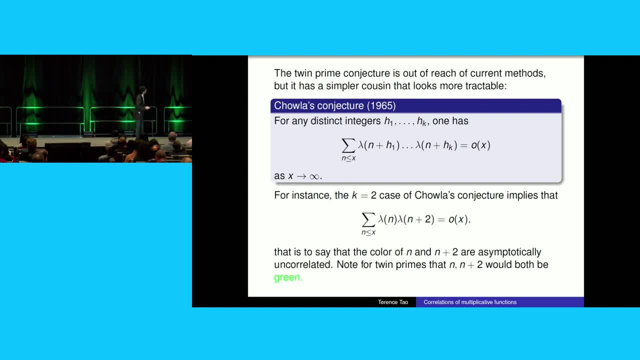 of the twin prime conjecture, where you don't work with primes but you work with red and green, And that's called the Charler conjecture. So rather than okay, so the general case, let me start with the special case. 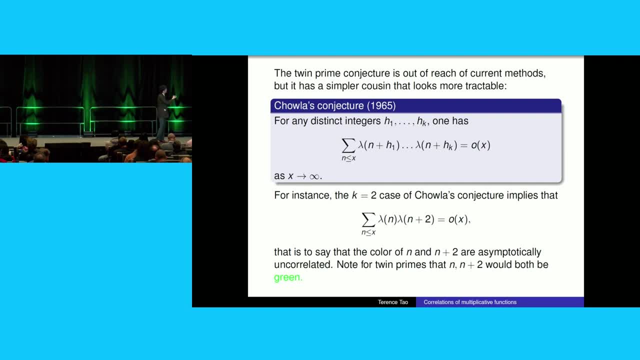 So, instead of looking at twins and n plus 2, which are both prime, you just look at n and n plus 2, and you look at whether they're red or green. Okay, so we know that n is red half the time. 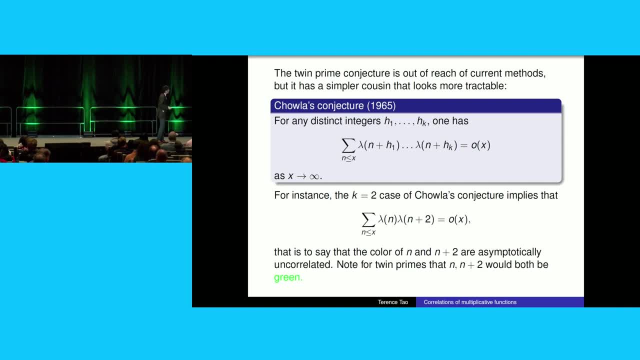 green half the time. n plus 2 is red half the time, green half the time. But the expectation- and the numerics support this quite strongly- is that they aren't correlated. There's no relationship between the color of n and the color of n plus 2.. 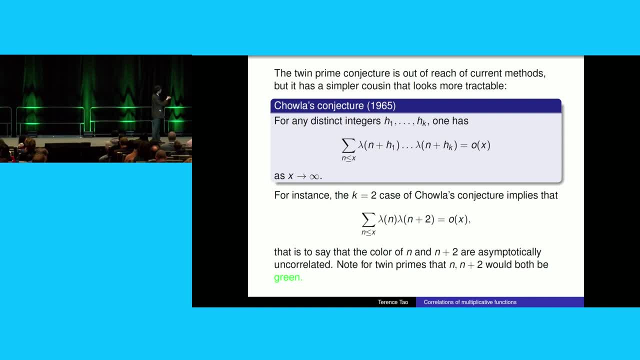 And the way you write that mathematically is that you look at the correlation function. You sum lambda of n times lambda of n plus 2, from n up to x. The trivial one by the triangle inequality is x, but that should be decayed faster than x. 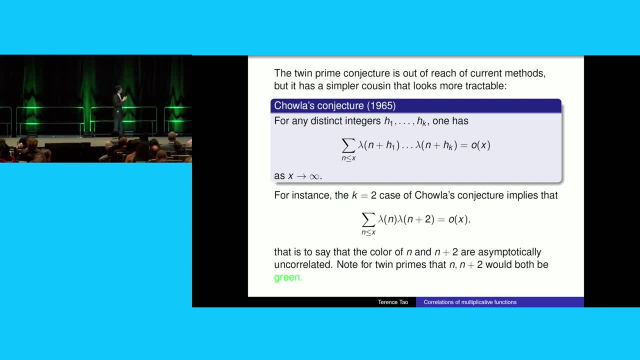 So asymptotically, on average that should be zero, If you like. that's saying that one quarter of the time and n plus 2 are both red, one quarter. they're both green, one quarter red-green, one quarter green-red. 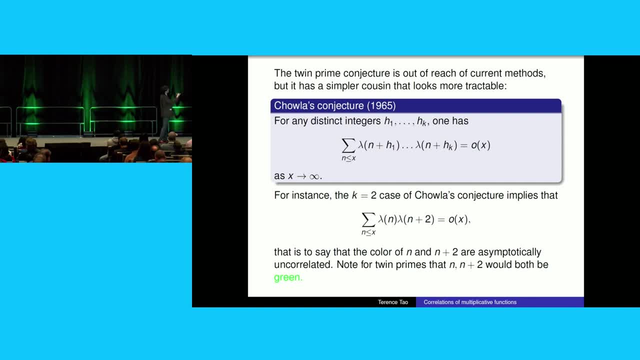 They're like independent, random variables. And then there's a k-term version where you don't just take an n plus 2, but you take k-term variables with different shifts of n and there's a very similar conjecture. Okay, So this is considered. 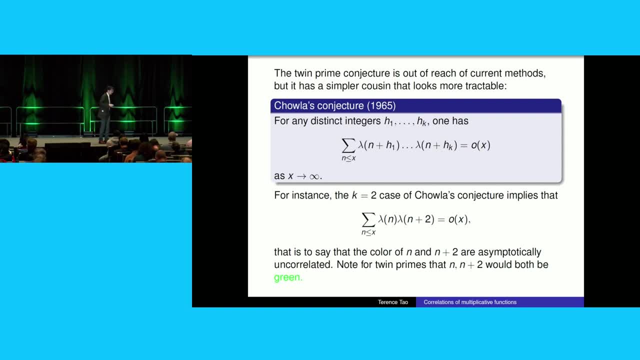 Well, actually for a long time this was considered the same difficulty as the twin-prime conjecture, but it was realized more recently that this is actually an easier. I mean, we can't solve. We still can't solve either. 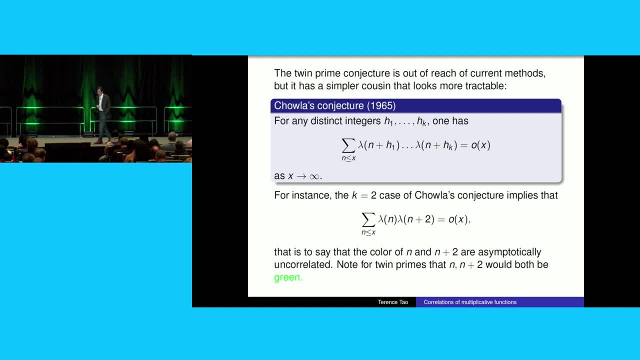 but we are closer to solving the Charler conjecture than we are to solving the twin-prime conjecture. I mean, the parity barrier is still mostly unbreached, but somehow the big wall is thinner here than it is elsewhere. Part of the reason is that, you know. 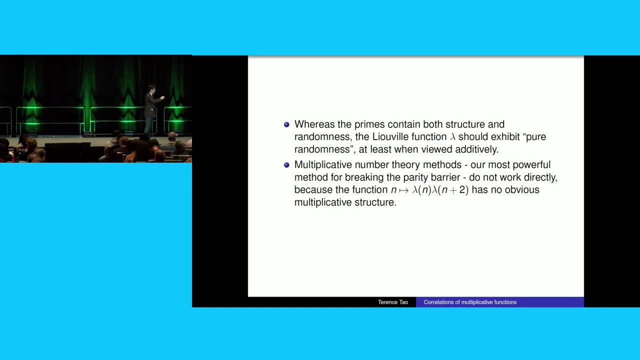 as I said, the primes contain both structure and randomness, and that's annoying. That creates lots of extra effort. Louvre function is kind of more like pure randomness. I mean, there is still some multiplicative structure and it is multiplicative. 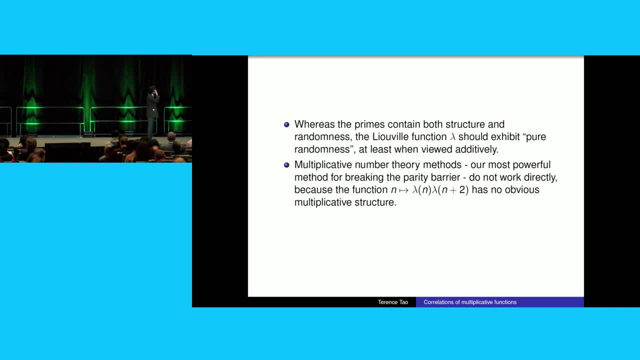 But additively it really looks like random noise. Yeah, so it. That's one reason why it's easier. The other is that it's not sparse. So our most powerful parity-sensitive method is multiplicative number theory, But unfortunately it doesn't work like. 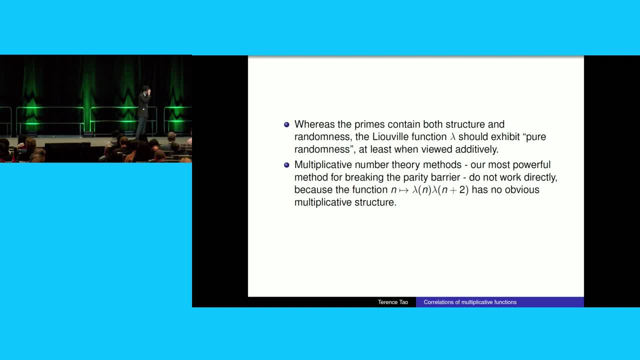 People have certainly tried. You can try to set up, you know L functions or Dirichlet series and so forth, but you run into a problem really early on in the process, which is that So lambda is a multiplicative function. 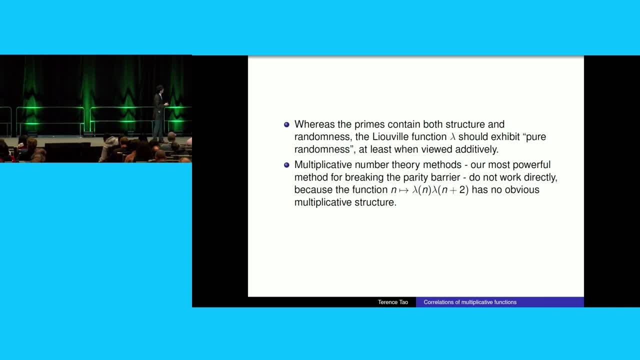 but lambda of n plus 2 is not, And so you know, this product of lambda of n plus 2, there is no relationship between its value at n, its value at m, its value at n plus m. There's no obvious multiplicative structure. 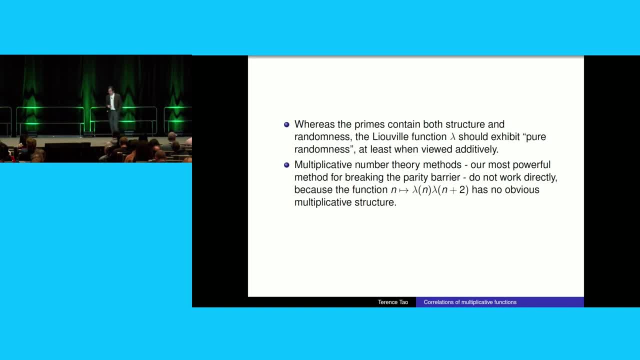 The shift by 2 destroys all the multiplicativity. So I mean you know it's still got factors that have multiplicative structure. so you know, but it's somehow buried And it's, We can still access it. 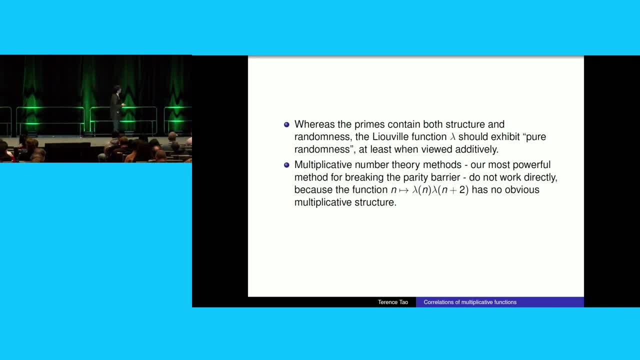 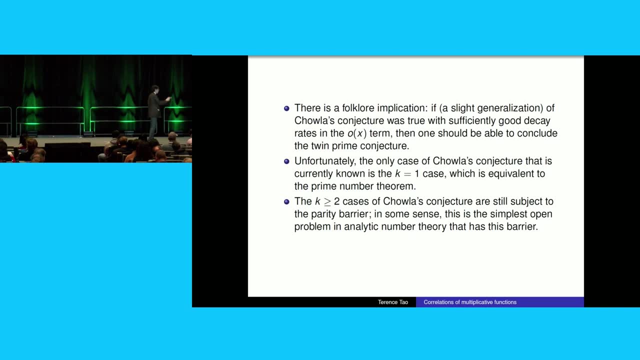 We've been able to access it sort of indirectly and we'll talk a little bit about that, but we cannot run the prime number theorem argument. It is not equivalent to 10 primes and there's no. They're not exactly related. 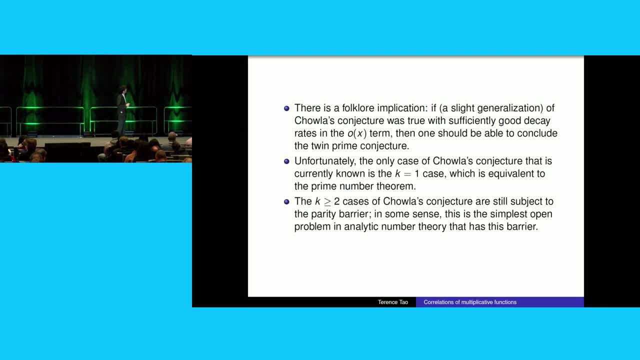 There is a focal implication which no one has actually bothered to write down. Maybe someone should at some point- that if you can prove the Charley conjecture but you have to prove a more general version which is technical, You have to first of all get better error terms. 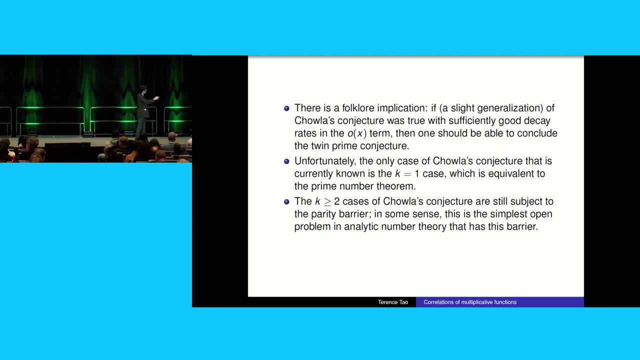 in the literal of x, and you also have to have some more coefficients and you need some uniformity in the coefficients and there's a lot of technical caveats. that's probably why no one's ever written it down. But if you can prove a sufficiently strong version, 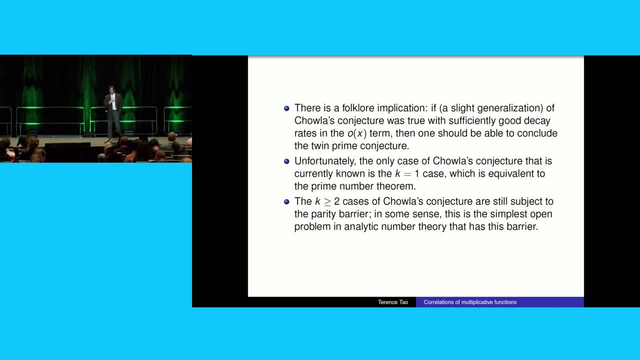 of the Charley conjecture, then that's I mean basically, once you break this wall somewhere, then all the other techniques. It's like this big dam of water. This parity barrier is like this dam. There's this huge body of water. 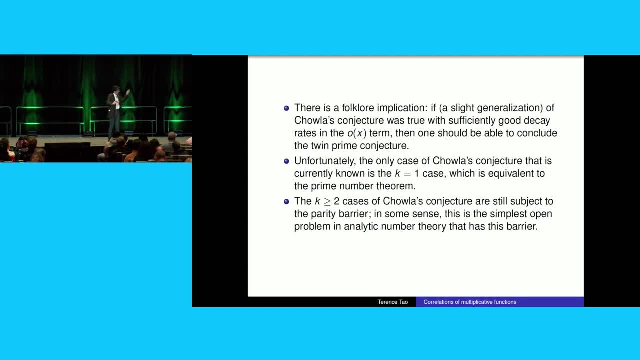 All our I think number of things are just waiting to be used to solve things beyond the barrier. but we don't have a breach. But once you have a Charley conjecture, that's a breach in the barrier. There's some ways to convert that. 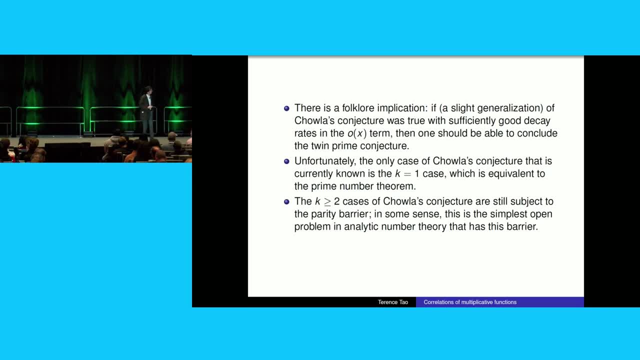 to then attack other problems that were previously out of reach. So yeah, if you can prove a sufficiently strong version of Charley's conjecture, then you should also be able to attack 10 primes and things like that. But we can't do that. 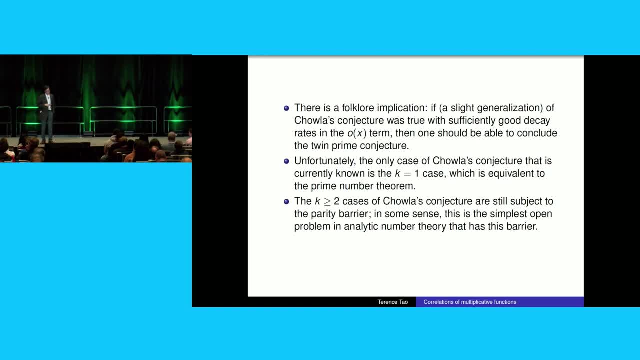 In fact, technically, as stated, the only case that we know is k equals 1, of one function, which is the Pi number theorem. But 2 and higher are sort of the easiest unsolved cases And we've been able to make some progress. 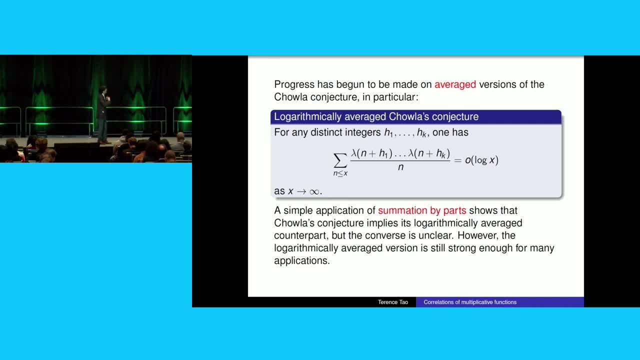 Yeah, so there's this technical thing. So traditionally in number theory we take these what are called natural averages, We sum up to x and divide by x, and that's sort of classically what we've done. It turns out that there are: 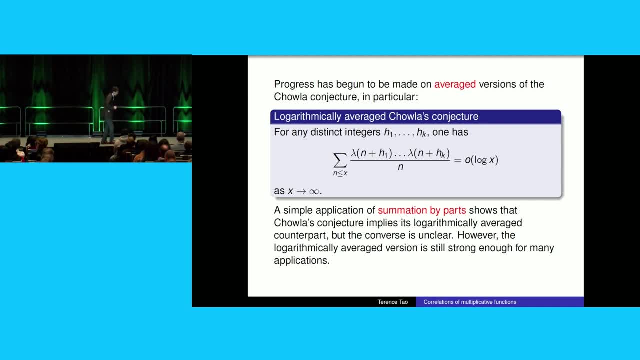 but it's a rough cutoff at x and it creates some technical issues. So there are gentler ways to sum. I mean you may know of Chouzao's summation of summing series that are divergent And there's something kind of similar in number theory. 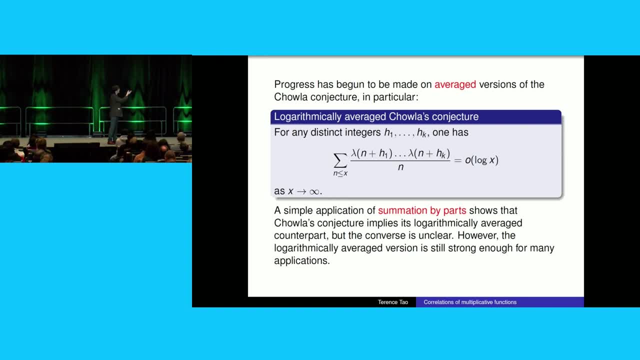 It's called logarithmic averaging. So instead of summing whatever you want like sum of lambda n plus h1 up to lambda n plus h2, unweighted, you weight by the harmonic weight 1 over n and you divide, you sum up to x. 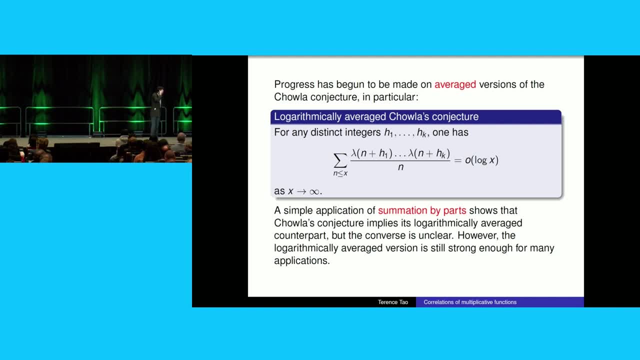 and you divide by 1 over log x And this is a better weight. It's closer to being multiplicatively invariant. So natural summation has got nice translation of invariant properties. I mean uniform measure is a translation of invariant measure. But as you know, on say the positive reals. 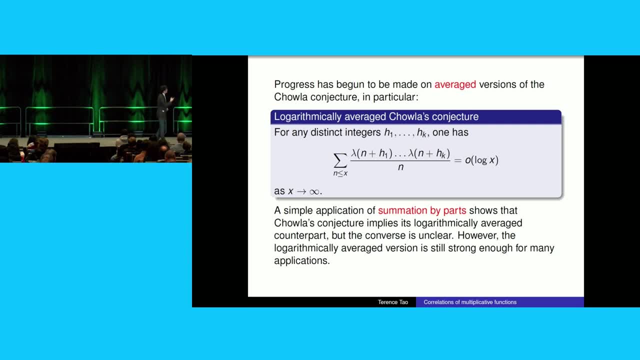 dt over t is a multiplicative, invariant measure. This is discrete. It's kind of like a discrete multiplicative almost high measure, Weighting by the integer of 1 over n. it's not a high measure but it tries to be. 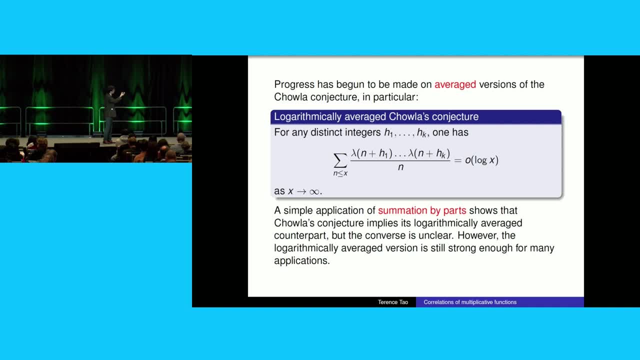 And because there's still some multiplicative structure residual in this problem, it is convenient to do this averaging. So there's this average version of the conjecture which is weaker. There's an easy summation by parts argument that if you can prove the original Chalice conjecture, 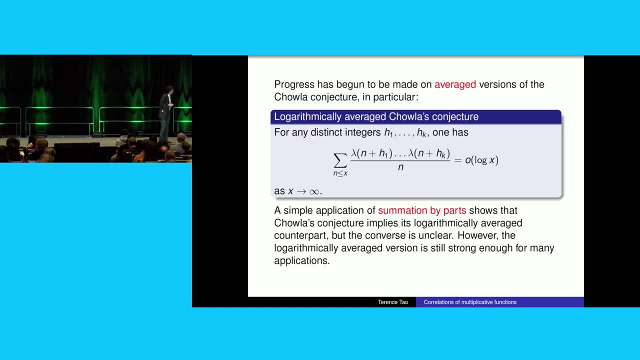 with no weights. you can prove it with this logarithmic weighting. It's kind of like if a sequence converges, then it's a series converges, then it also chiseled converges. It's a very similar type of argument. 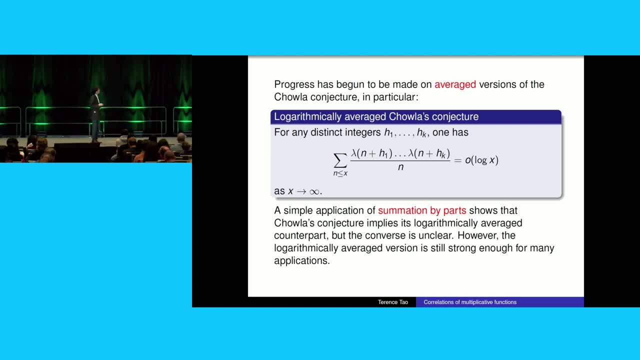 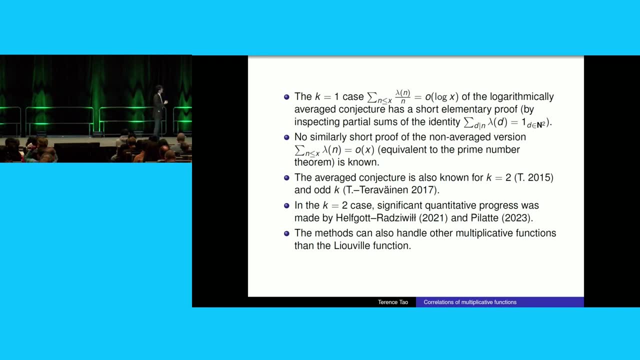 But not. conversely, This is strictly an easier problem. So just to illustrate this, so, as I said, if you want to control the natural averages of the Louvre function, that's as hard as the Prandtl number theorem And there's still no really short proof of the Prandtl number theorem. 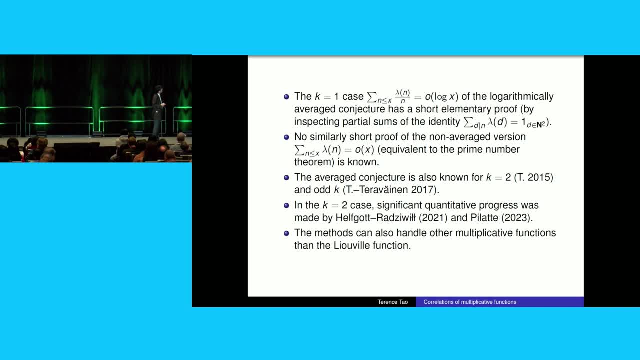 But if you want to control just the logarithmic averages of the Louvre function and get some cancellation that you can move from half a page. It comes from a very simple identity that if you sum the, if you take a number n and you sum all the Louvre function of all the divisors of n. 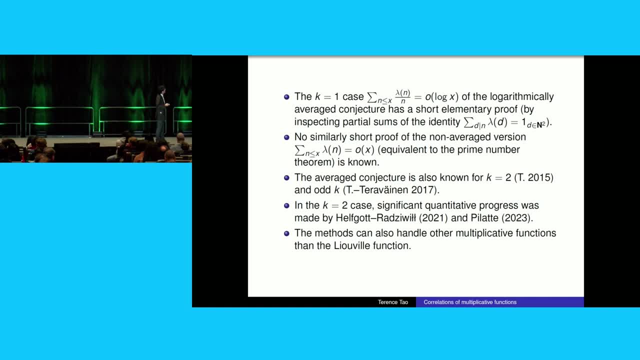 that turns out to be one when d is a square and zero. otherwise That's a nice identity And you sum that for d up to x. you very quickly get this identity, this estimate And this log average thing. we can actually prove some cases. 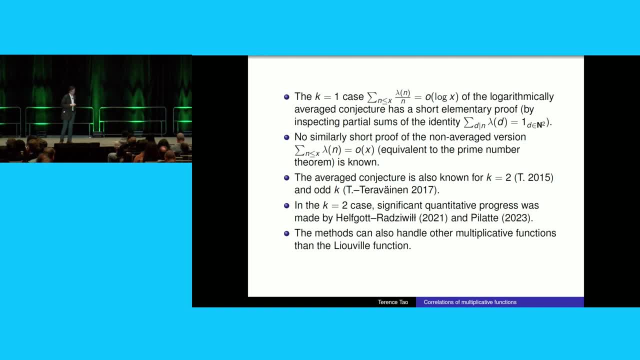 So a few years ago I was able to prove the log average version of the Charley conjecture with k equals 2.. And then with Yoni-Tervainen we were able to also get the odd case which, unfortunately- I mean that sounds like we got half the cases. 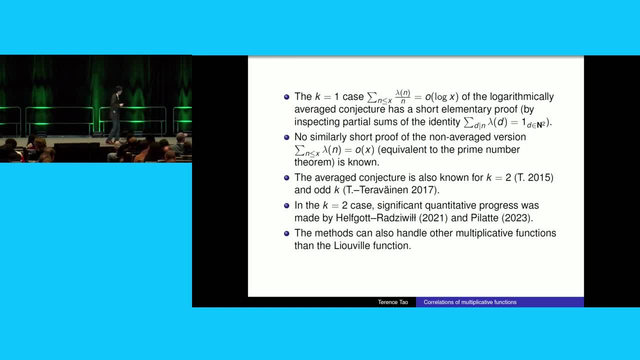 but actually the cases that are all the most useful are the even cases. If there's some positivity, that is really helpful. But we could get the odd cases at least. And then recently the quantitative version, the bounds on the k equals 2 have become extremely strong. 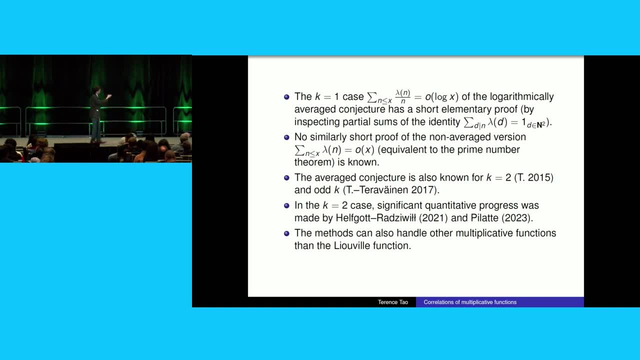 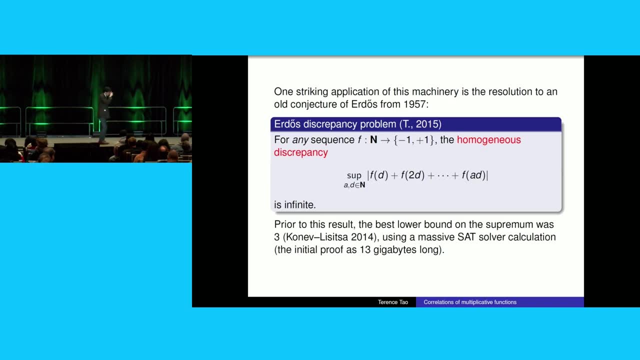 surprisingly so, actually, And we can handle not just the multiplicative Louvre function but many other functions like this. So one of the first applications of all this theory was that I was able to solve this old conjecture of Erdős, which is this fun conjecture about discrepancy. 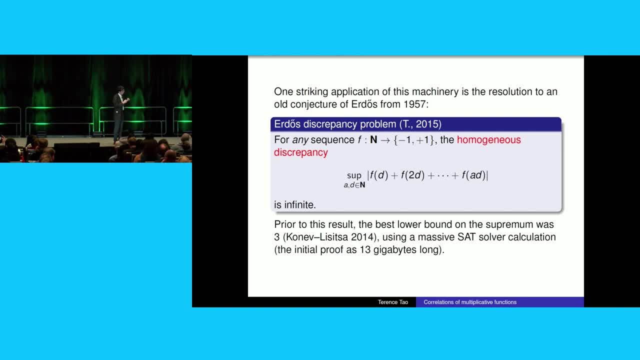 and discrepancy theory. So discrepancy theory. so it's asking: how well balanced can you make a sequence of plus or minus ones? You know there are Ramsey theorems that say that no matter how you try to distribute the plus minus ones evenly among natural numbers, 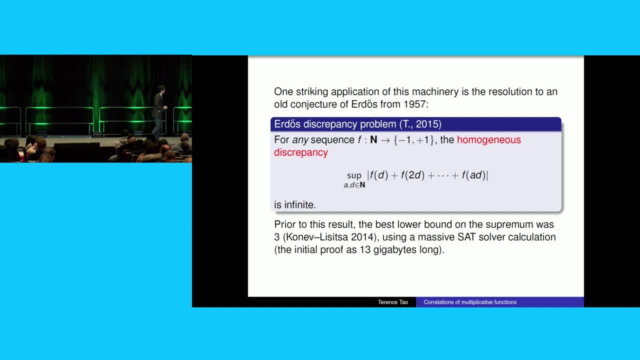 there must be some ethnic progressions where it's all ones, or some where it's minus ones, as the famous van der Vaarten. But Erdős asked: suppose you look at just what are called homogeneous ethnic progressions: D, 2D, 3D, up to 80,. 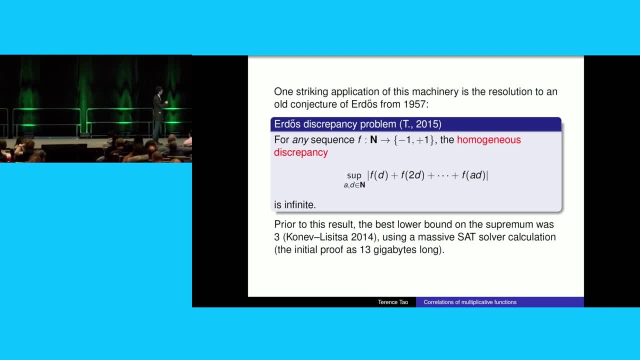 progressions where the spacing is the same as the initial starting point And you just want to make your function balanced on these homogeneous progressions. Is it possible to find a function plus, minus ones where these discrepancies are all bounded? So is this the soup of all? this sum is finite or infinite? 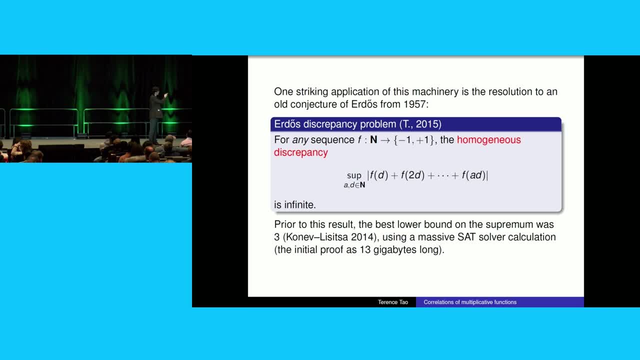 So I proved it wasn't possible, that it was that, in fact, this: that no matter what you did, this discrepancy had to be larger than any finite number. It was infinite. For comparison, the previous best known result was just one year previously. 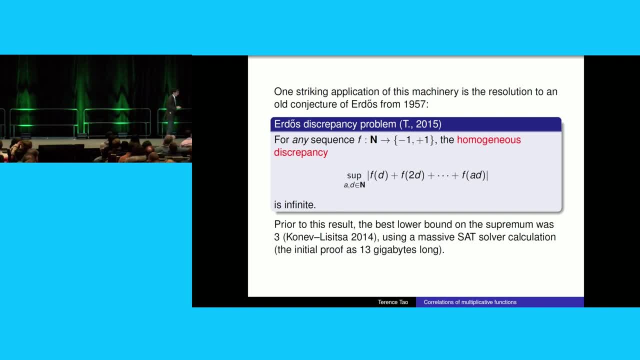 that we know the discrepancy was at least three. That if you color the natural numbers, there was some homogeneous progression where there were three times more plus ones than minus ones, or vice versa, And that was not an easy result. That used one of the massive SAT solvers that I mentioned. 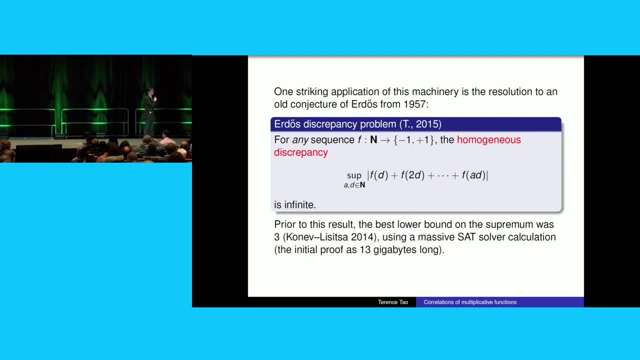 my first talk And at the time the proof was the longest proof, the largest proof ever created- 13 gigabytes, which is, but that's now like a 10,000th of the largest proof. I think there's a petabyte proof out there. 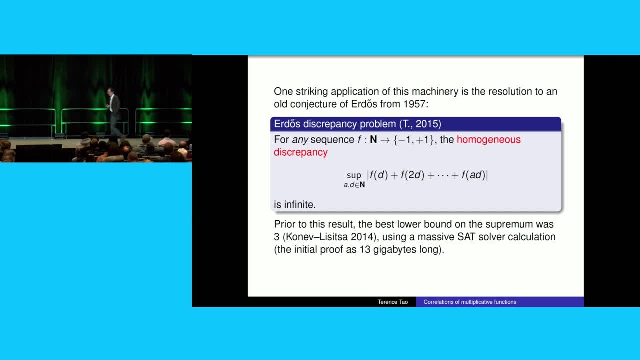 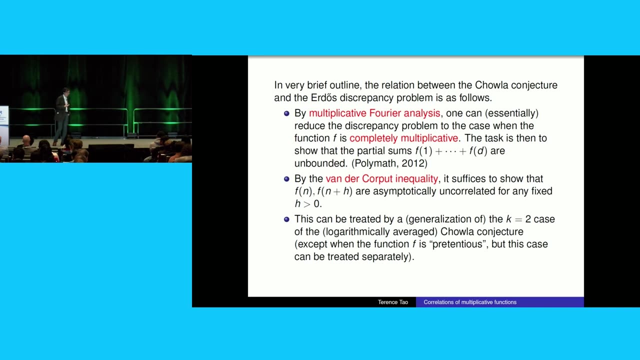 But at the time, in 2014, it was- it was briefly held the record of the largest proof. I'm not going to say too much about the, how you reduce the, how you derive the discrepancy problem from the Charlec conjecture. 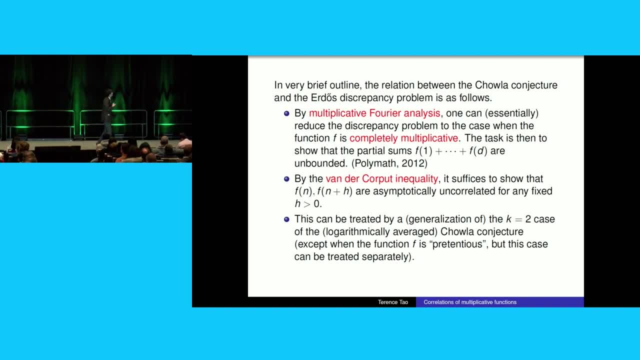 Well, I'll just say in very, very high level. So this, the Erdős discrepancy problem, concerns an arbitrary sequence of plus, minus, ones with no multiplicative structure. But you can do some multiplicative Fourier analysis and there's a reduction, Roughly speaking. you only need to understand. 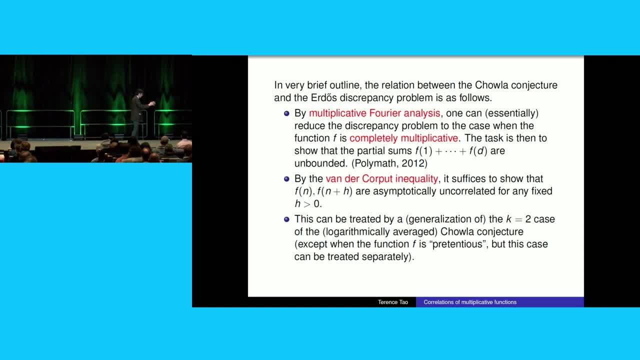 what happens for multiplicative sequences, And if you can do that, you can derive what happens for arbitrary sequences with a little bit of Fourier. It's a little bit of Fourier analysis magic. And then- and the advantage of doing that is that these 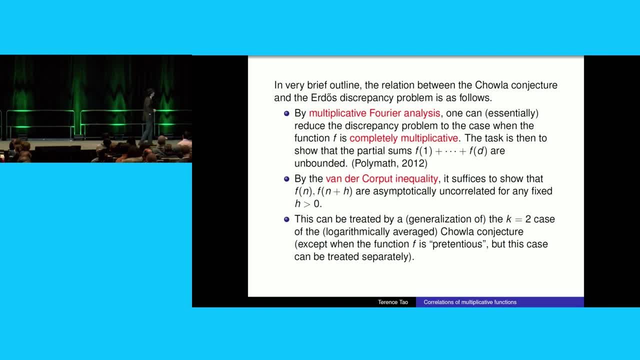 these sums over homogeneous progressions just collapse to partial sums, And then so you just need to show that the partial sums of certain multiplicative functions are unbounded with some asterisks that I don't want to talk about, And there's a standard. so this is a global sum. 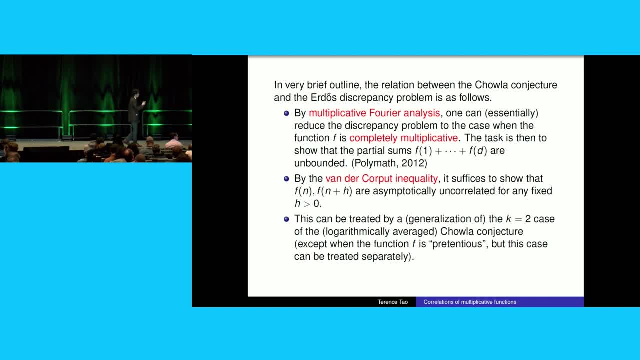 a long sum. but there's a standard trick to control global sums by short sums. It's called the Van der Koopa inequality And basically, if you want to show that that a long sum gets bigger and bigger, it just needs to show that adjacent numbers. 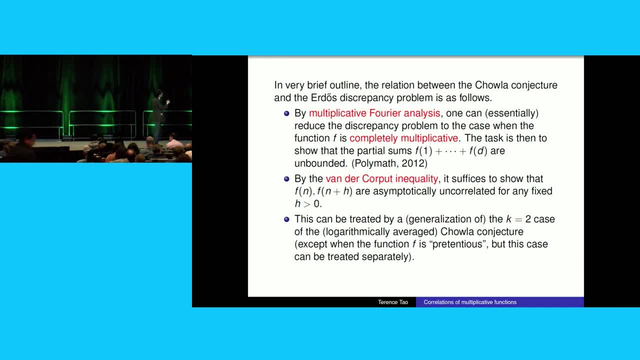 are not correlated very much. So you can reduce things to understanding the correlation between adjacent or nearly adjacent values of this function f, And that's basically the child conjecture, And so you can use progress in the child conjecture to solve this problem. 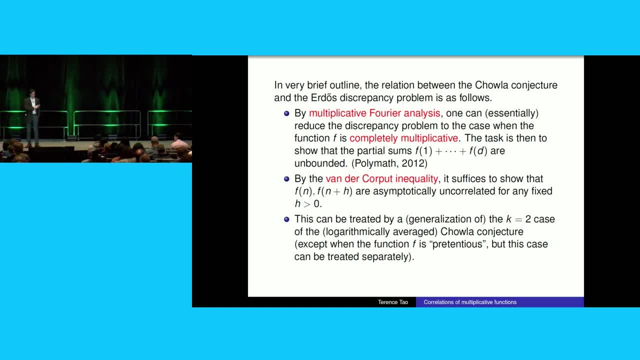 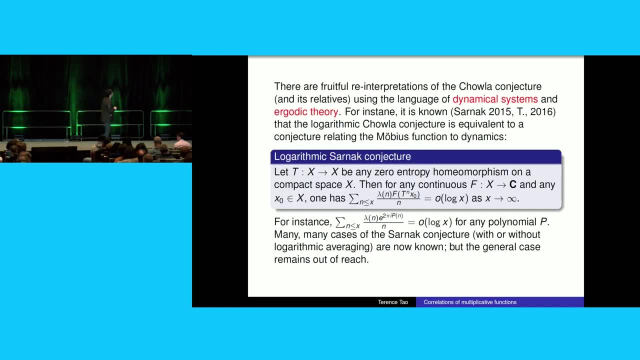 Again, there's an asterisk. There's some functions for which the child conjecture doesn't apply, ones that are functions that are called pretentious, And that's another great story. I can't talk about it. All right. So there are all kinds of areas of mathematics. 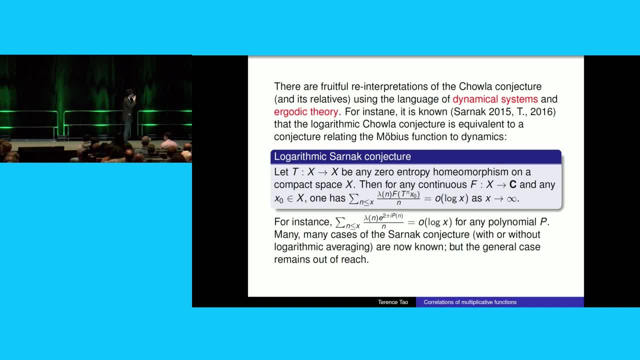 So I won't talk about it so much. but it is also connected to a conjecture in relating, or in some sense not relating, the Louvre function to dynamical systems. So one way to formalize the fact that the Louvre function is somehow random is that it should not be. 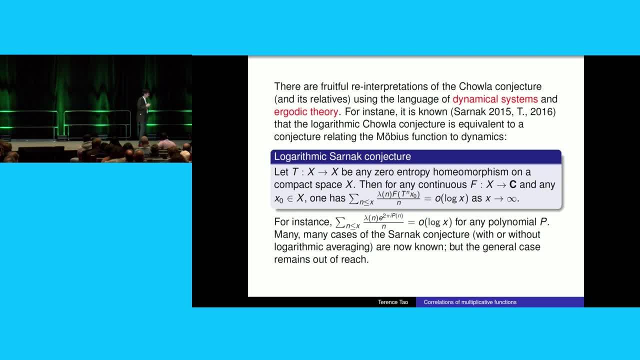 there should be no way to even approximately predict it using some kind of predictable sequence. So there's this notion in agonic theory of something called the 0.6 sequence. It's a sequence which is generated by you have some dynamical systems. 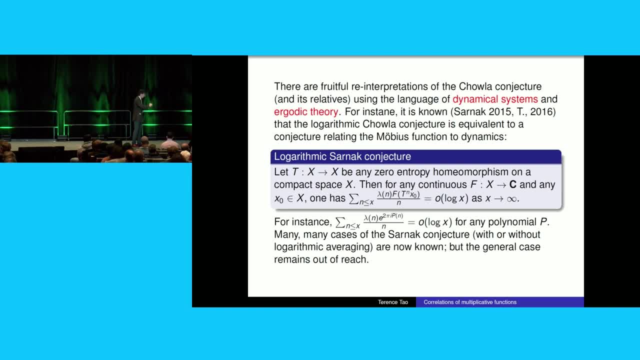 some compact space with a shift, and you take an orbit and you divide your orbit into two sets and you put a plus one in one set, the orbits in one set, minus one in another and you get a sequence of plus minus ones. 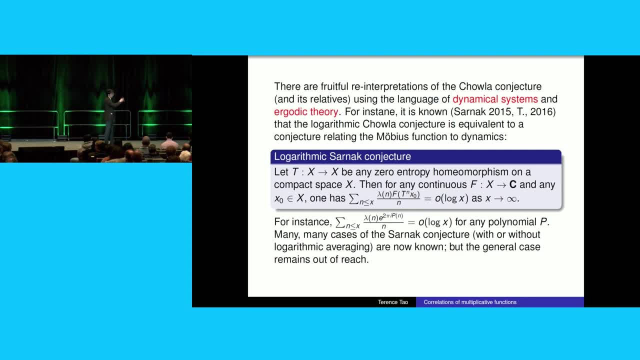 Now, every sequence of plus, minus ones can be generated by in this manner, from some dynamical system, But if you restrict to a very rigid type of dynamical system what I call the zero entropy which I want to define here, 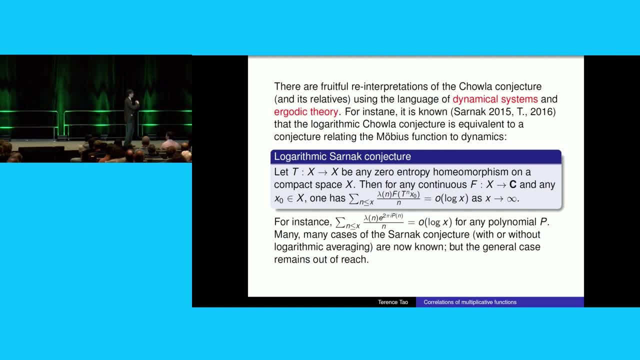 then the sequences you get are very rigid. You get things like periodic sequences or almost periodic sequences, Or, for example, e to the 2 pi i has a polynomial of n. It's a very typical deterministic sequence And there's a conjecture of Sarnak. 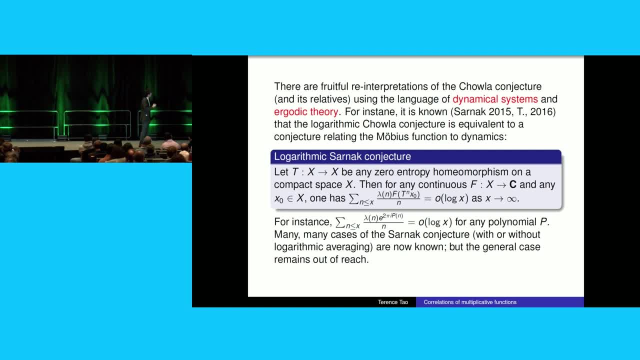 which, roughly speaking, says that the Louvre function is uncorrelated with any deterministic sequence. So basically, no, yeah, if there's a sequence which doesn't generate much entropy with much randomness, then it has nothing to do with. 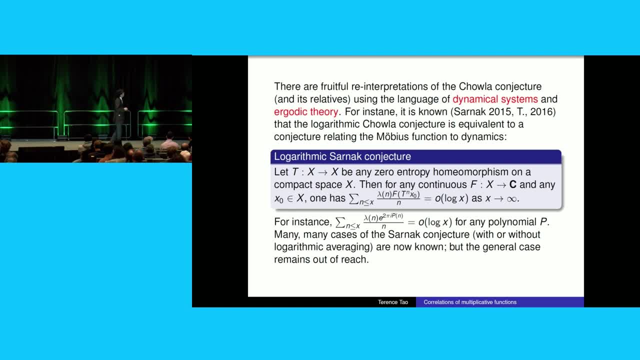 asymptotically with the Louvre function, And that turns out to actually be equivalent. it's a different way of expressing randomness, but it turns out that it's equivalent to this Charler conjecture, at least with this log averaging asterisk. 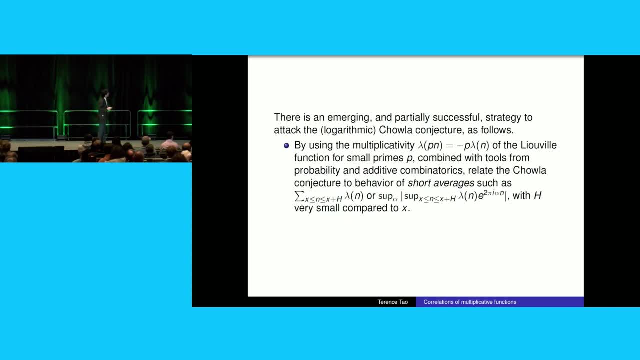 But maybe I will not talk about it more. Yeah, so we would like to settle the Charler conjecture. for many reasons It would settle this Sarnak conjecture as well. We would stop being able to attack many other questions about multiplicative functions. 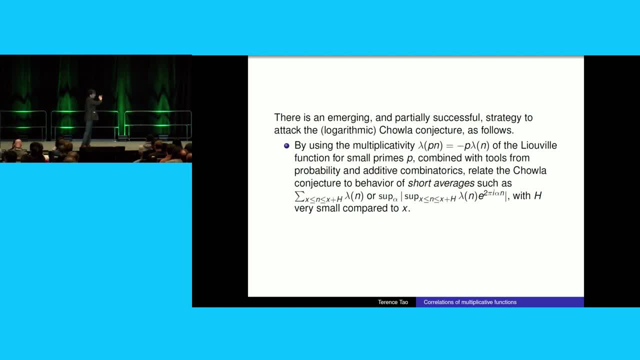 And already the progress we already have has settled some old conjectures already. Well, we saw one, but there were several others And maybe, as I said, in the future, maybe we can start attacking trim primes and all the other things on the other side of the parity barrier. 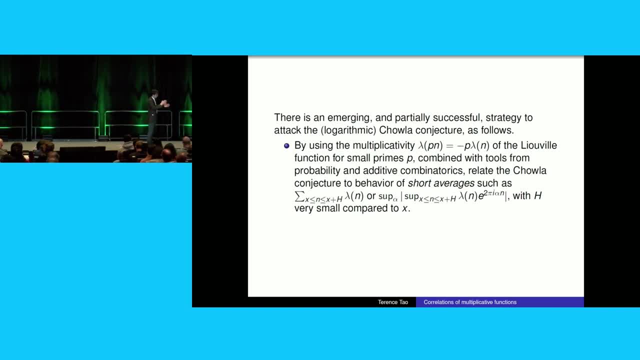 And we are sort of getting close. It's like this barrier has got like several layers to it And we've managed to break through some of them, but this was one last barrier which still completely has no crack in it, But somehow exactly one breakthrough away. 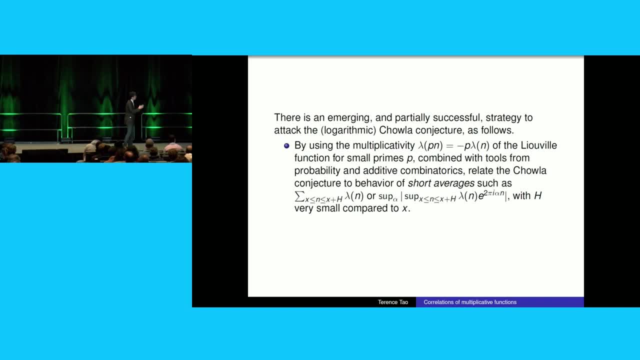 from really having a great theory, as opposed to five breakthroughs. So we do have a strategy to attack this conjecture now in general And it's based on. So we are largely exploiting the multiplicative structure, as I said, of the Louvre function, especially at small primes. 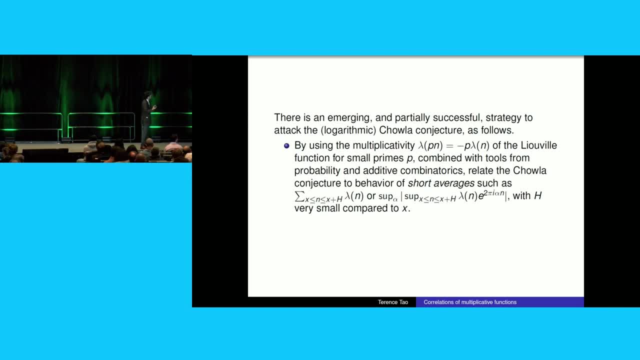 So the Louvre function is multiplicative. So one consequence of this is if you multiply n by a prime, it flips the color. So if you multiply a red number by p, it becomes green and vice versa. So lambda of p is always negative of. 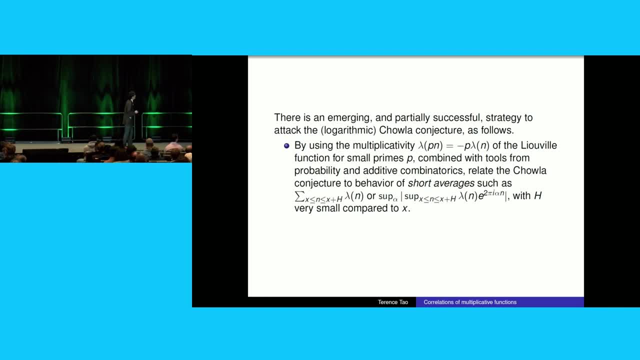 That p should not be there. It should be negative lambda of n, not p times lambda of n. And so every time you want to correlate, say n and n plus 1 or n plus 2, you could try to dilate by p using the complicativity. 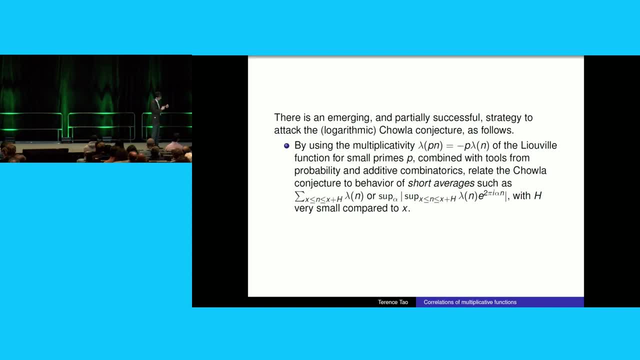 And now, instead of looking at the correlation of two nearby numbers, you can look at the correlation of two almost nearby numbers. Now that seems a bit worse, so you can further away now, But then you can try to play games like you try to average in the prime. 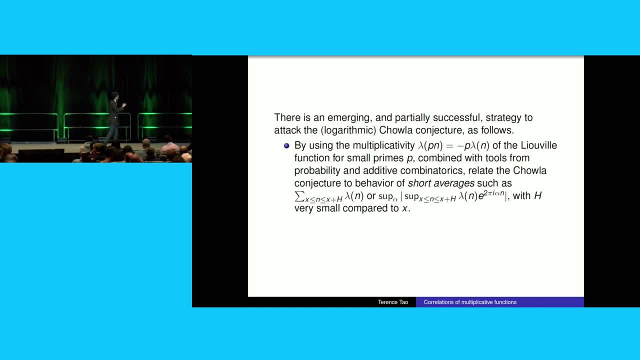 And that You know the more averaging you have, the better chance you have of getting some cancellation. And so you want to relate these short, these very local averages to slightly longer-range averages, And so we were able to do this, and we're able to do this in a way that's not so much. 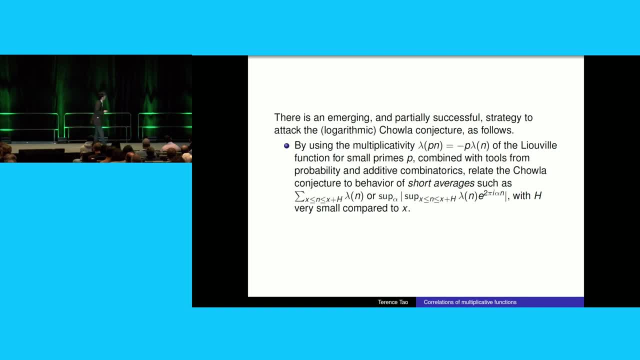 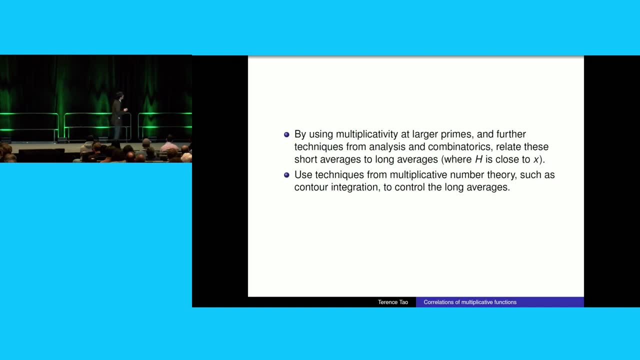 to the extent There are certain short-interval averages that we can relate effectively to, say the two-point correlation of the Charler function or k-point correlations. So we can kind of inflate the our scale of averaging a little bit. On the other hand, if you've already 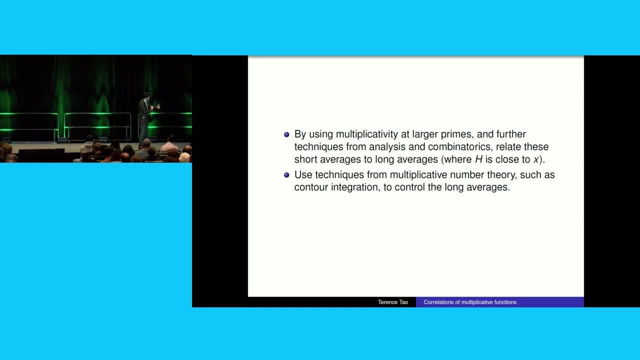 if you already can, if you already got to the point where you're studying averages on a somewhat long interval, then you can use the multiplicative again, And there are ways to inflate the long interval to ones on even longer intervals, Again using multiplicativity. 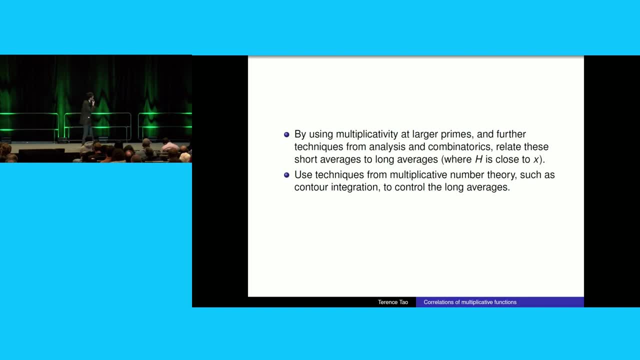 And a bunch of techniques from analysis and combinatorics. graph theory shows up a lot, And so you can try to inflate things And, once you're on really long averages, when you're averaging a function on really long averages, finally multiplicative number theory becomes very useful. And you know the prime number theorem kicks in. You know, if you have the Riemann hypothesis it becomes even more useful. But even without the Riemann hypothesis you can get lots and lots of good bounds on long averages. 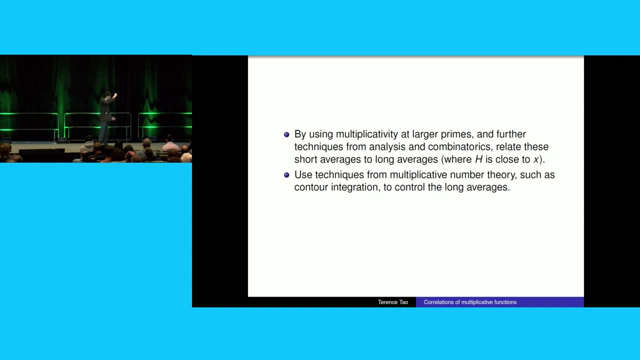 And so this is hierarchy of scales, And if we can just sort of get a complete chain from, you know, scale one, which is what we need to control, Charler to the larger scale, which is where multiplicative number theory works. 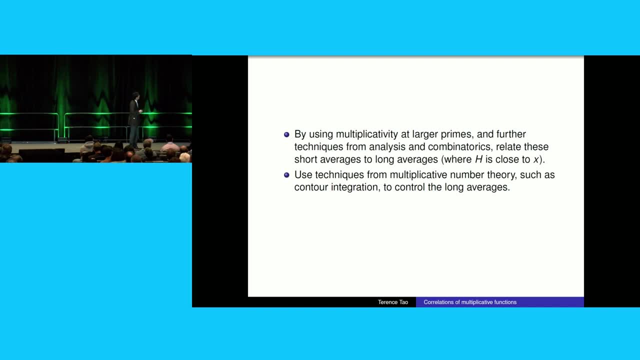 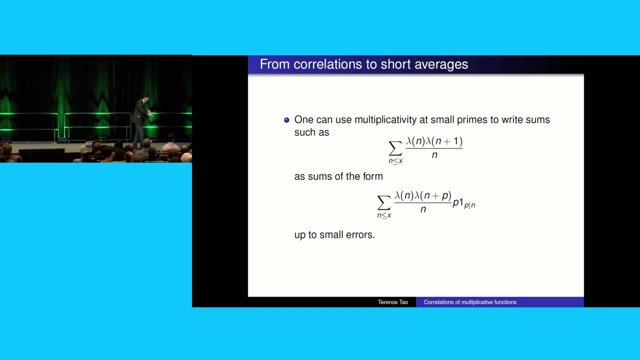 then we can actually do all this. So And we have like 90% of this chain complete, But this is a gap. So, as I said, you know, if you want to, for example, control the average of lambda, of n lambda plus one, 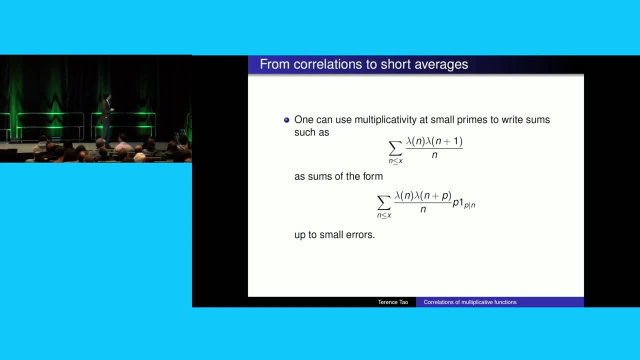 you can inflate it by p And you basically end up staring at correlations of lambda of n plus p. But this is one price you pay is that you have to restrict numbers n that are divisible by p, Otherwise there's no relationship here. 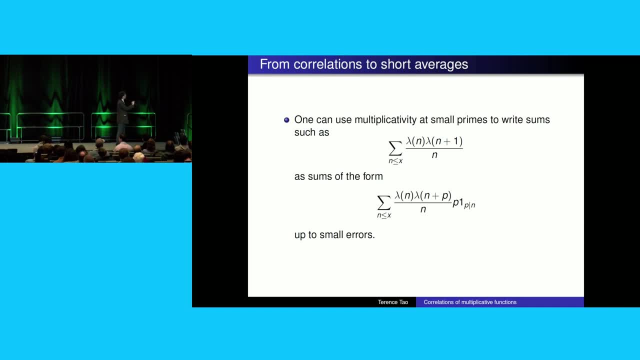 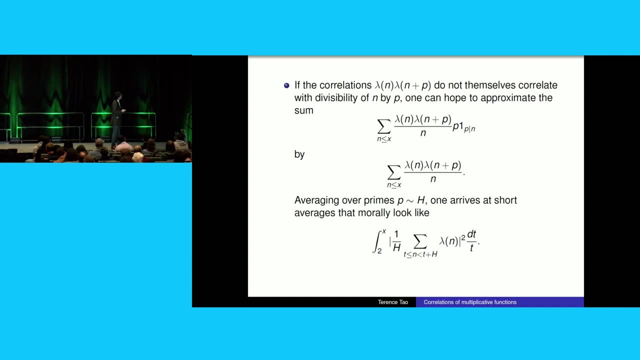 You see again, the weight one over n is not actually a hard measure. This is because of the discreteness. So this is divisibility by n which is annoying, But we have ways of dealing with, We have ways of removing this divisibility constraint. 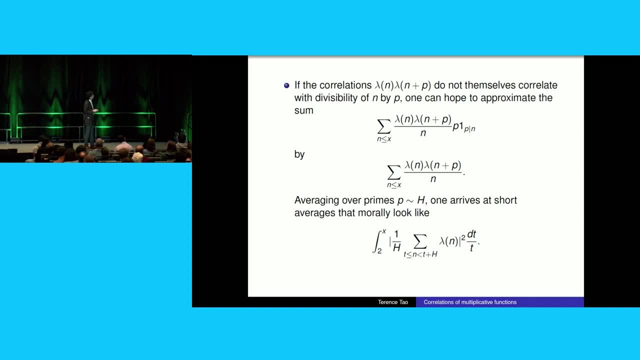 So I introduced a technique called. I introduced a technique based on information, variation and entropy, And then later introduced a technique based on expander graphs And so, But as long as you don't, As long as you keep the primes reasonably small and you work with small intervals, 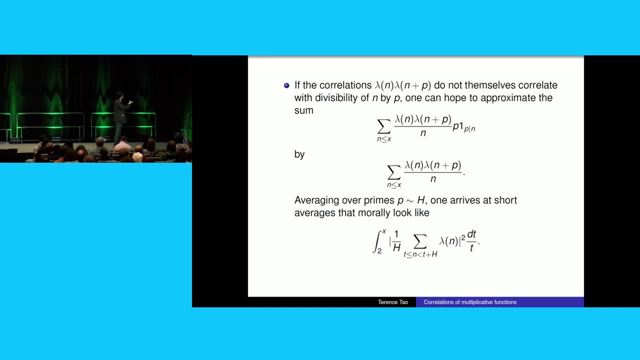 you can replace, You can remove this divisibility on p relation, and then you have an expression that is actually much more tractable, And then you average in p And then you basically are reduced to understanding short averages of this little function, And that turns out to be a problem that was solved. 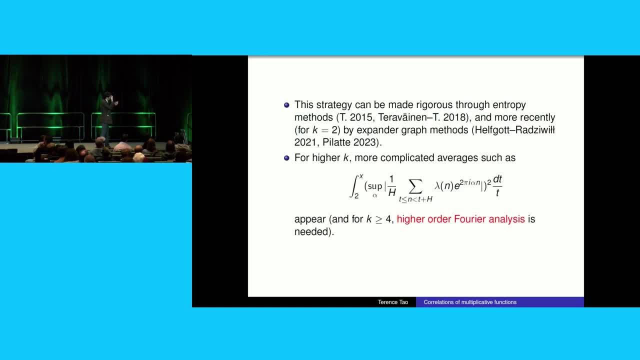 There was a breakthrough in Well, at least for two-point correlations. there was a breakthrough in multiplicative number theory, that by Matamaki and Matsui- that managed to somehow push the multiplicative number theory methods all the way down to almost scale one already. 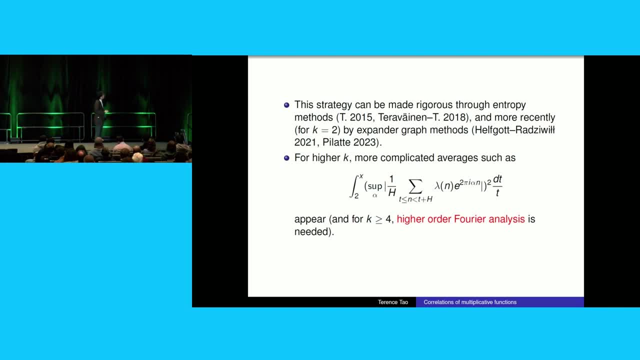 And then just by adding this extra little input you can get all the way down. So with two-point correlations it all works And you can get- And we have this two-point Charlotte For higher k- you can do some of this analysis. You could. You have to start inputting higher-order Fourier analysis, which is another great story which I cannot talk about, But it ends up You have to study averages, not of the loop function directly, but loop function twisted by various phases, like twisted by a linear phase in the simplest case. 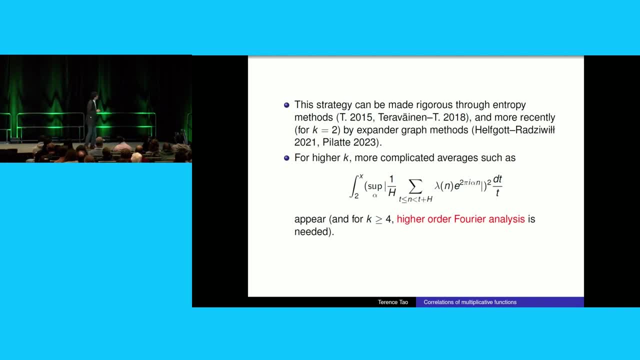 K equals 3. And then it gets a lot worse for higher k And unfortunately that breaks the multiplicativity. And now the Matamaki-Urasi theory does not extend to meet these averages. But we are able to relate, Charlotte, to sort of small scales. 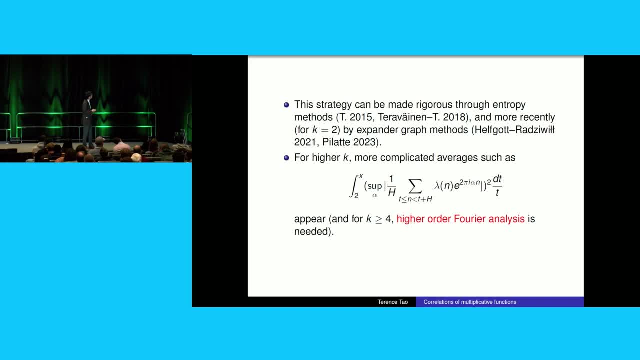 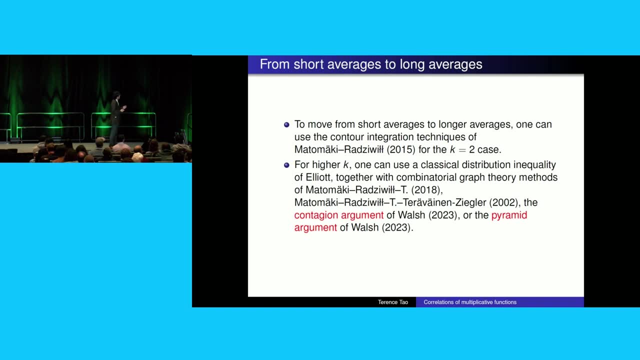 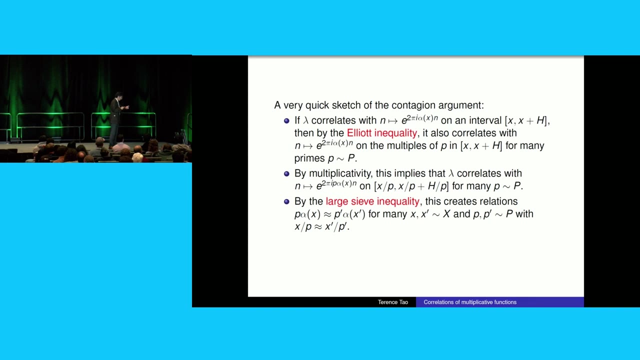 Short averages of scales less than log x. roughly we can do, Yeah, So yeah, I think I will skip the slide. Let's see How much time do I have actually Right, Okay, So we have a separate argument. 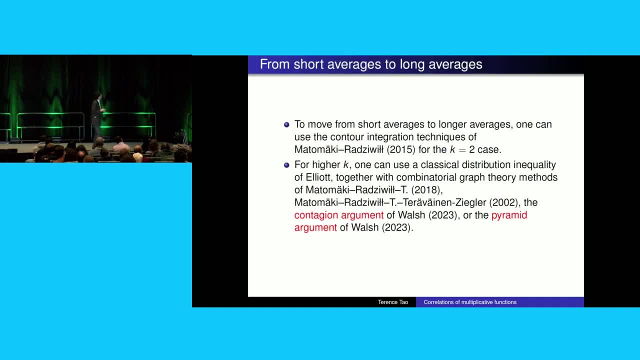 So we have actually multiple separate arguments. But there's a lot of very exciting progress by Walsh, who introduced a bunch of really elegant arguments which can relate reasonably short averages to long averages. So there's one argument he has in particular called the contagion argument. 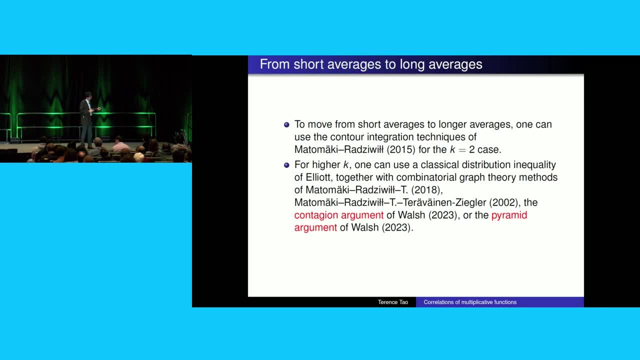 So if you want to show that on many, many short intervals the loop function behaves randomly, So you assume that it doesn't Okay. So you assume that for many, many short intervals the loop function is doing something non-random. For example, it's oscillating at some frequency here. 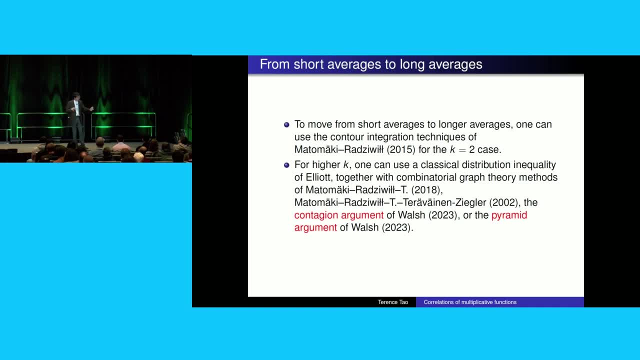 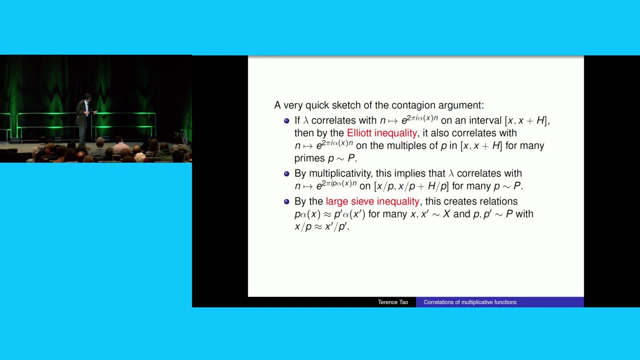 and over here it's oscillating at some other frequency and so forth. So there's lots of intervals that are somewhat infected with some Fourier frequency. Now it turns out that, because the function is also more applicative if you take an interval and you dilate it by a prime, 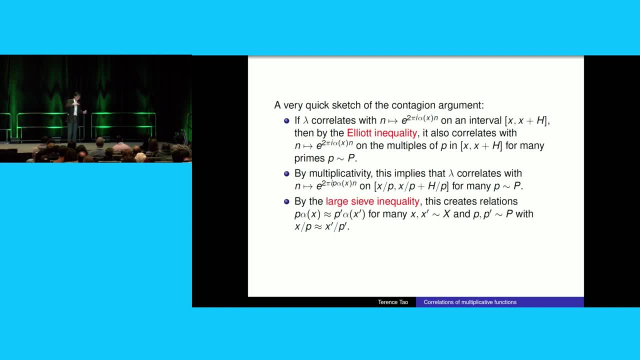 if you're already oscillating with some frequency down here, the dilation will probably also be oscillating with some related frequency up here, And then if you undilate it somewhere with a different prime, it means that at different intervals, probably the frequency that one interval oscillates at 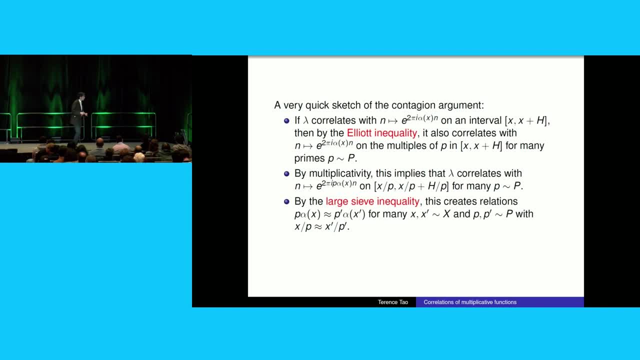 and another interval that oscillates at they're related And using a bit of graph theory, you need the fact that the operation of multiplication by primes and division by primes kind of creates some sort of expander graph And you can show that once you force a little local correlations. 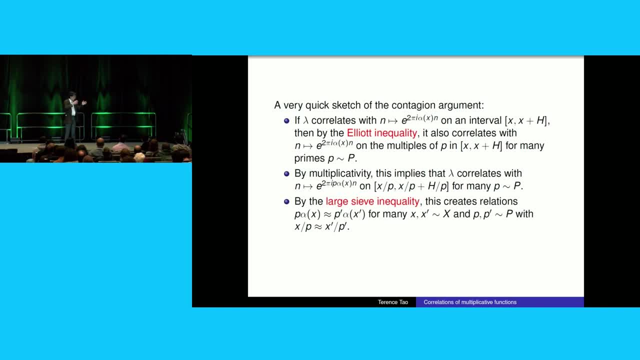 in your loop function. you can kind of glue them together and they infect the bigger intervals, And these slightly bigger intervals also must also start exhibiting some oscillation at certain frequencies, And you can keep chaining this in a big pyramid and you can eventually get a very big interval. 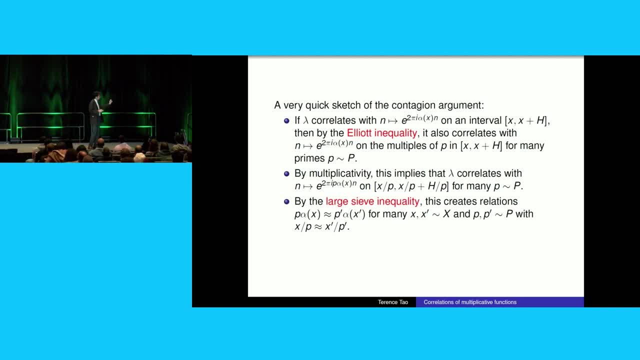 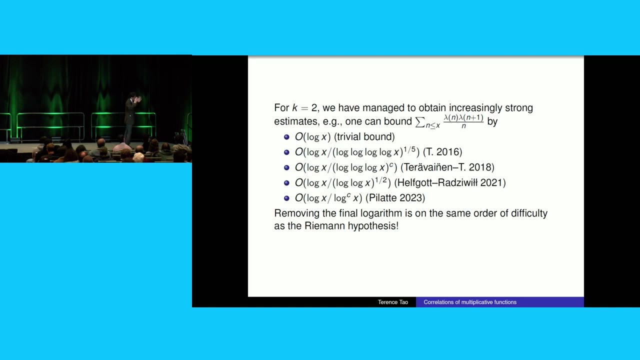 where there's a very big oscillation which you can rule out by multiplicative number theory. So there is a strategy, There are ways to make this all rigorous. I think I will skip the actual details. And all this theory works beautifully in two points. 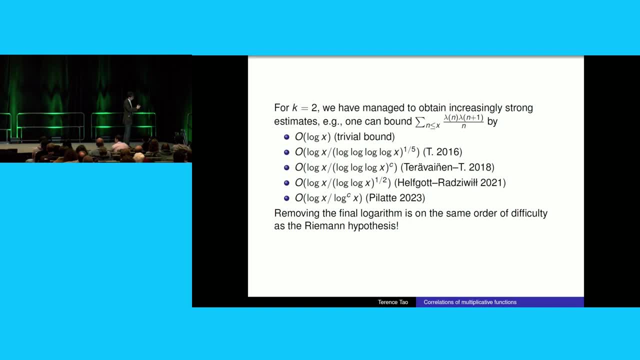 For two points. there's no Fourier frequency at all. You just have to average the plane loop function, either weighted by one or by a digital character. It's all very straightforward, And so for two points, we're getting it. I mean, the theory is simple. 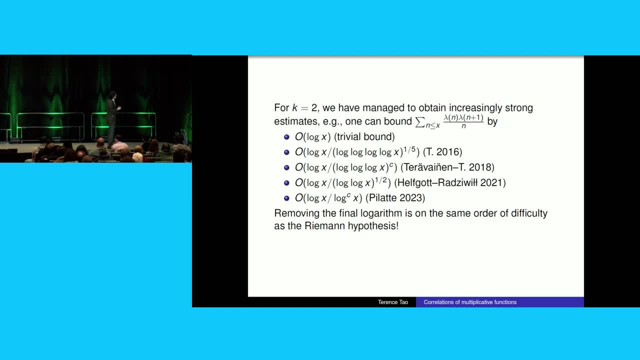 It's just that it's become extremely satisfactory. So, for example, you want to control log averages of lambda and fs1, which is the kind of thing you need to solve the discrepancy problem. The trivial bound is log x if you just take absolute values. 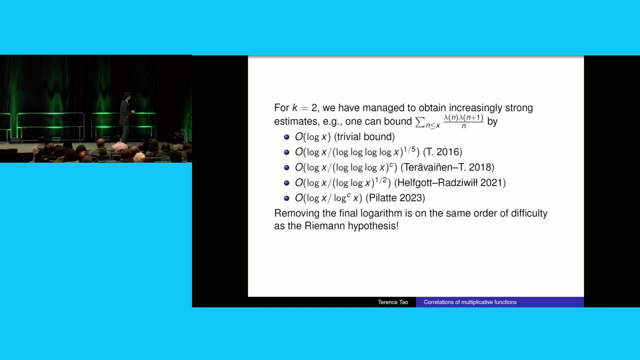 You know I was first able to get little of log x. I could get a tiny decay. I eventually went back and actually tried to figure out exactly how much decay I got in that argument and I got a very tiny amount of decay. 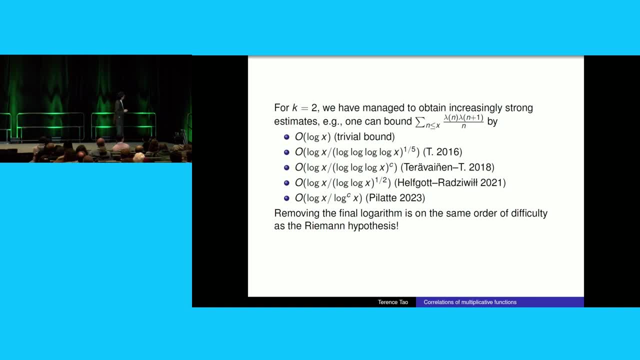 I could gain basically four logs of x. There's a standard joke that I think number theorists. what does the drowning number theorist say? This is log, log, log, log, log. We have a lot of logs in this business. 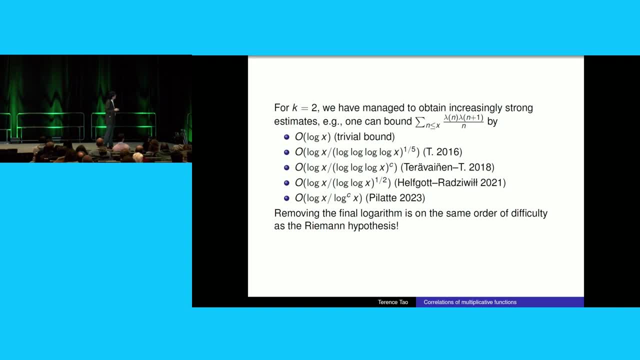 But over time the arguments got refined. So with Yoni we managed to optimize the entropy argument and get down to three logs. But then Hofgott and Radzoui used some very nice analysis of random walks on expander graphs which gave a significantly stronger result of log log x. 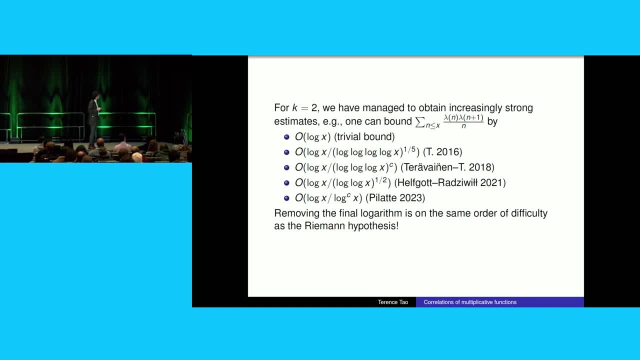 And just very recently there's a result of Cedric Pallat which actually even gets, you know, gets the gain down to basically one log, which is really quite amazing. You know, the next step would be to get a power saving. 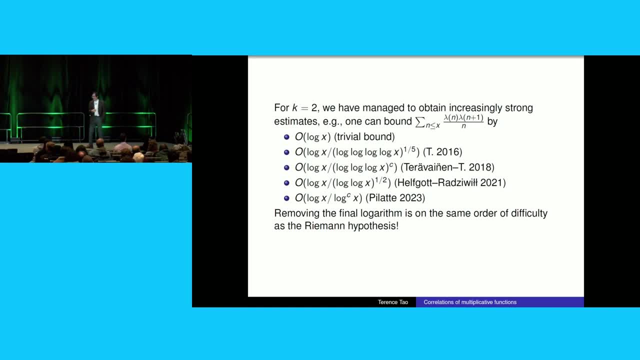 which is actually what's conjectured, but that's at least the Haas-Riemann hypothesis. So this is pretty much the best you could hope to get with all that technology. So we understand two-point correlations extremely well. now, In the odd case, there's a parity trick. 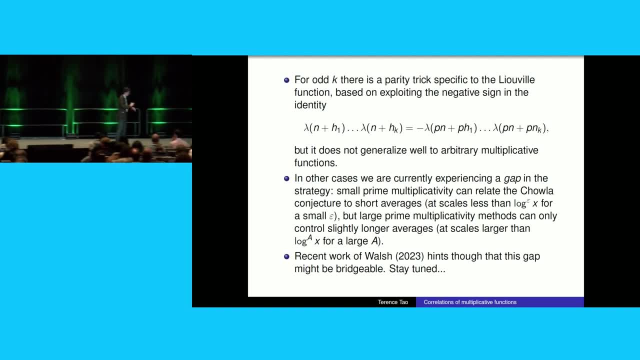 You may know, sometimes when you integrate by parts, like a trig function and exponential function, sometimes you can't quite evaluate the integral, but you can somehow show that it's equal to the negative of itself by like two integrationary parts and then you can say it's zero. 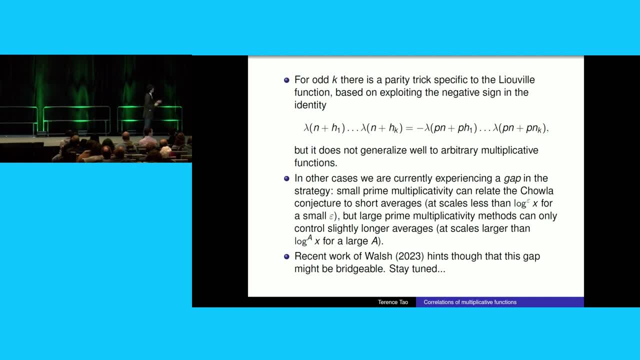 So there's a similar trick that lets you cheat and deal with the odd case somehow by dodging the actual difficulty, But it only works for Louisville and it only works for this odd case. And it's a pain, because the even case is the most interesting. 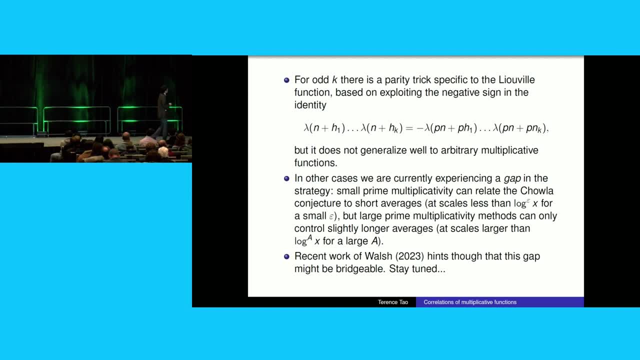 The even case implies the odd case, but the odd case does not imply the even case. Yeah, but we have this strategy. We can inflate short charler-type correlations at the micro scale to these sort of mesoscale correlations at log x with small power. 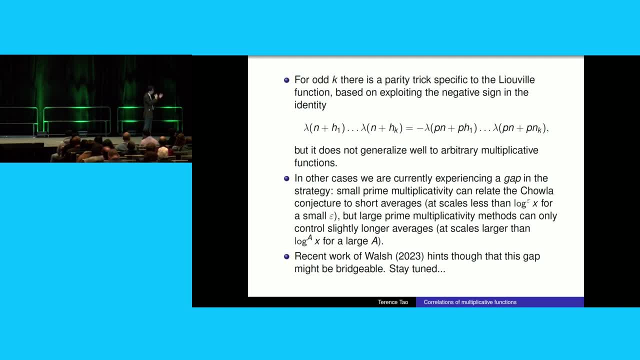 And Walsh has been refining his arguments quite a bit and in his most recent paper he showed that, assuming the Riemann hypothesis, which at this point we're willing to do- he can control averages even at scale log x to a large power. 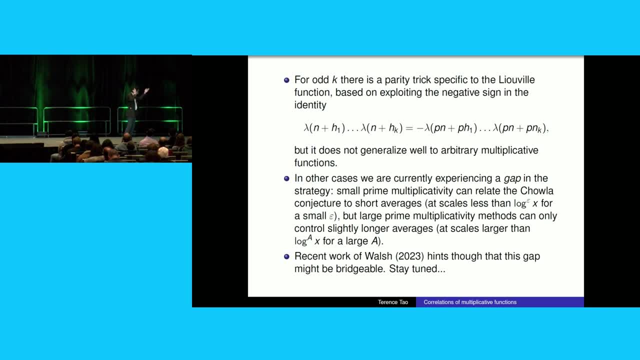 Log x to a is actually he can run his argument and control those averages by extremely large averages which we know how to control, And so we can get from the larger scale down to log a to a big power, and we can get from log a to a small power down to charler. 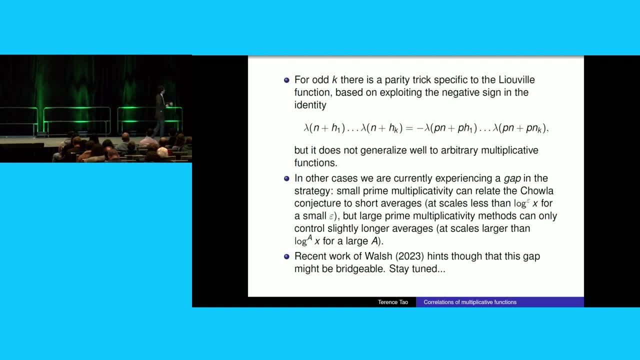 And this is one tiny little gap remaining- how to jump between log x to a small power and log x to a big power. And that is one thing where all our techniques break down for different reasons, But the log x I mean. it appears to be the fundamental barrier here. 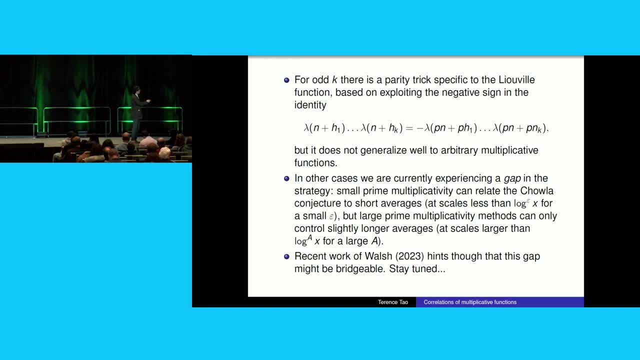 One reason is that the number of the product of all the primes up to log x is less than x. but it is a natural barrier for trying to use when you're trying to combine many, many primes together. But the most recent paper, Walsh. 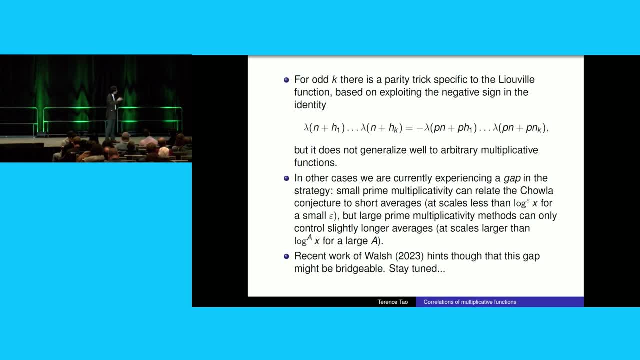 he has some intriguing hints that maybe his method can actually get past this barrier. He hasn't actually quite done it yet. I'm sure he's hard at work, But yeah, so basically stay tuned. I think there will be more progress in this area. 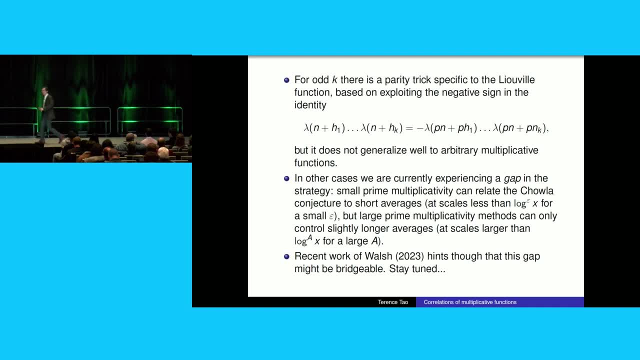 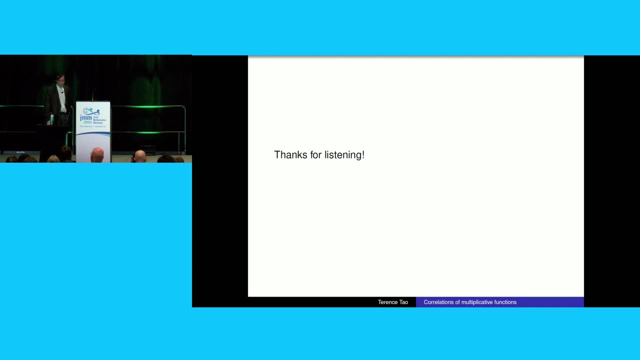 in the next few years. I think I will stop here. Thank you very much. Thanks very much, Terry, for a beautiful talk. We have time for some questions. There are two mics in the middle. Hi, wonderful talk. Thank you very much. 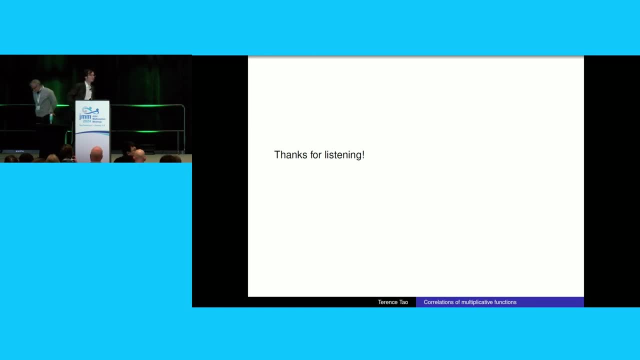 I just wanted to check on one detail. at the very beginning of your talk You mentioned that a certain asymptotic for the lambda function was equivalent to GRH. Did you mean GRH for cyclotomic fields or the entire GRH? No, just the GRH for Dirichlet L functions. 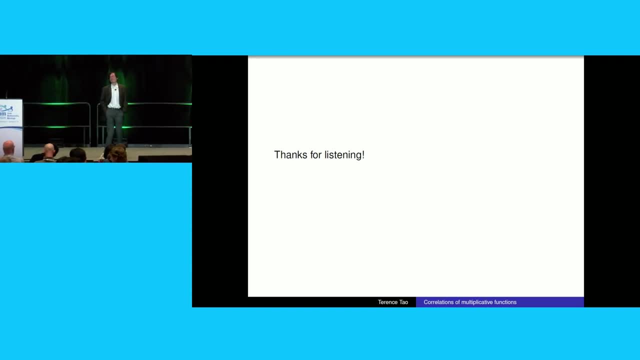 Okay, good, Yeah, you could probably write down an equivalent form for more general L functions. I haven't thought about exactly what it would be Okay, thank you. Hey, thanks for the talk. I just had kind of a naive question. 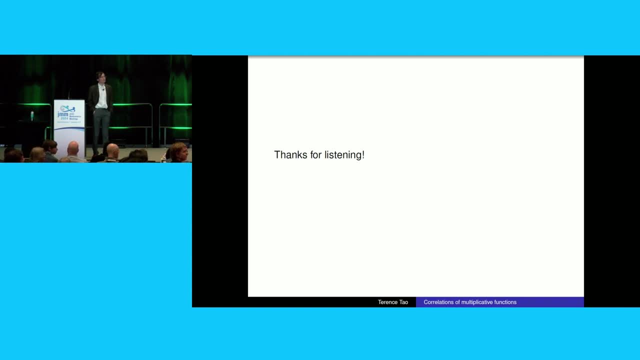 You talked about, I guess, methods that were parity sensitive, I guess just in analytic number theory. So there's like this fabled parity problem. And you also talked about the centrality of methods from multiplicative number theory and kind of like bridging this parity problem. 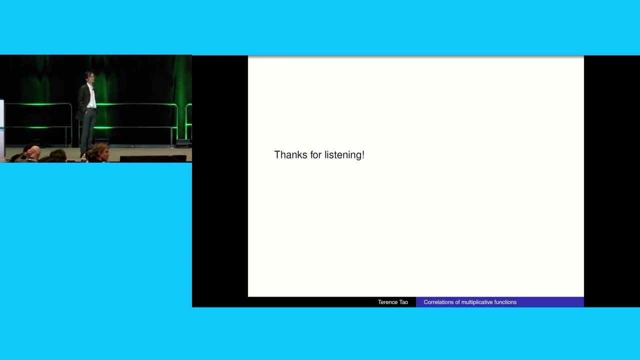 So I wanted to know were there. could you give an example of like a parity sensitive method that is somehow not from analytic or multiplicative number theory? Okay, so there's a small number. So methods from Ramsey theory are parity insensitive. So, for example, there's this famous thing with Zameretti. 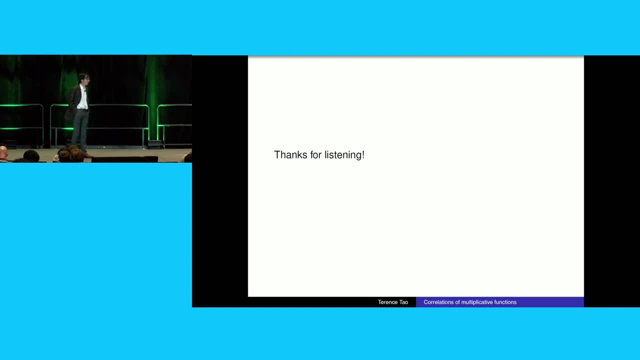 that dense subsets of the integers contain lots and lots of rhythmic progressions. And even if you delete half the integers, as long as somehow it's still dense in the other half, you would still get lots and lots of progressions. So it turns out that using tools like Zameretti's theorem, 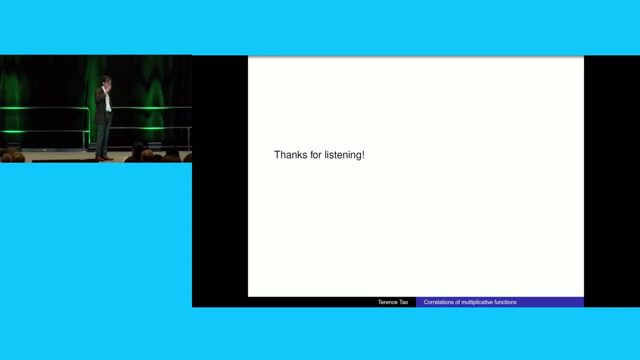 is somehow parity insensitive in some sense. You lose a factor of two or something, but you still get a lot of progressions. And many, many years ago I proved to Ben Green that the primes contain many arbitrary long arithmetic progressions And that was a problem subject to parity barrier. 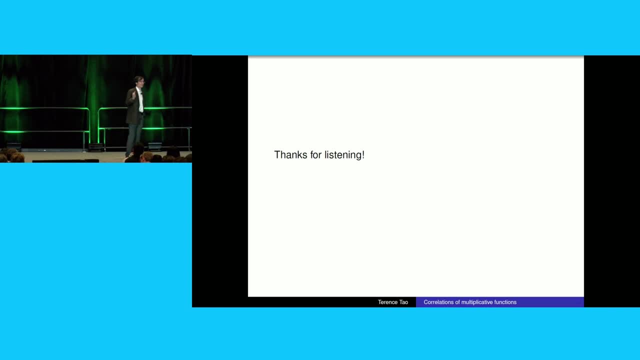 But because we used Zameretti's theorem, we could get around that barrier. Later on, we found another way to prove it, using many things, but including multiplicative number theory, and so we found a different route. Yeah, there are what are called bilinear methods. 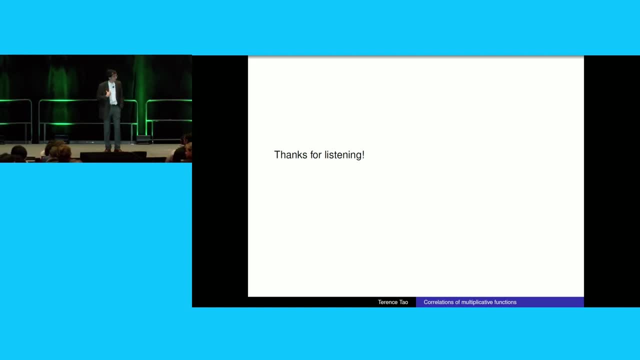 Yeah, so this parity barrier kind of blocks you from any technique that's based on sort of linear sums where you're just summing over one n and lambda of n times something. If you can somehow control bilinear sums where you have two variables, n and m. 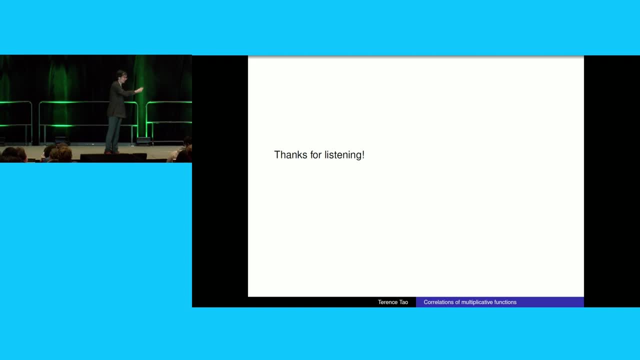 and you're summing some lambda of some polynomial of n and m times some weight. once you have two variables you can use, your weights might be able to distinguish red and green of the pair, And so, in the few cases where we can prove, 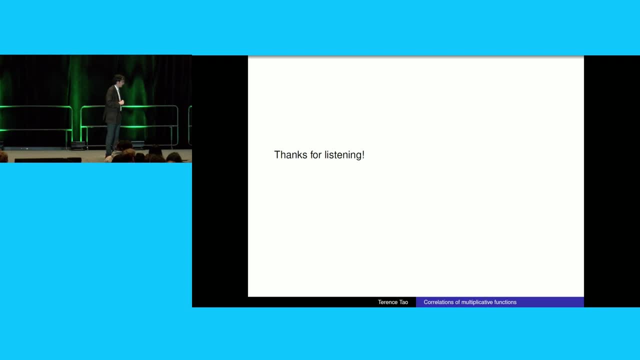 some bilinear estimates you can actually beat the parity barrier. So there was a celibate that was out of Friedland and Ivanić that you know. so there's this famous that there are infinitely many primes of n squared plus one. 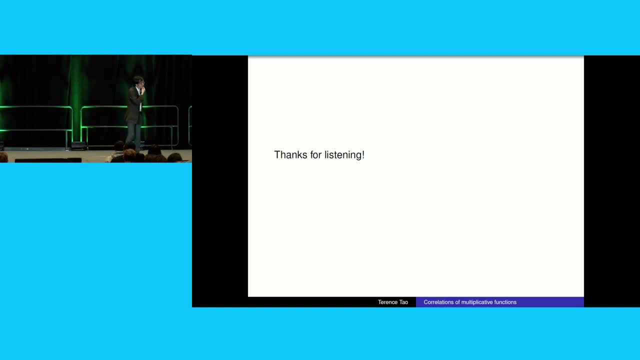 And we can't prove that because of the parity barrier. But Friedland and Ivanić showed there's infinitely many primes of n squared plus m to the fourth, which is a larger set, still very sparse. But there's certain bilinear sums involving n squared. 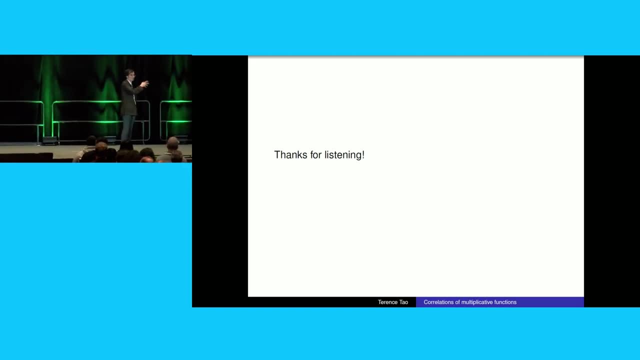 and m to the fourth, that, through the magic of algebraic number theory, they were able to get some handle on. It's a great result. Yeah, so there's a small number of times when we've, you know, breached the parity barrier, but very. 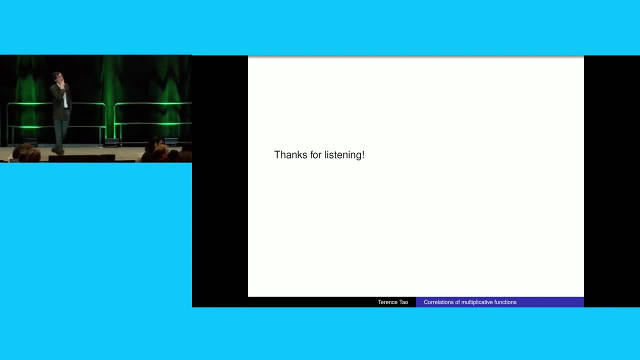 but they're still very rare. Thank you. What is the largest pair of twin primes known so far? Oh, I have to look it up. I saw yeah, there are people who've sort of devoted their computers to searching for these things. 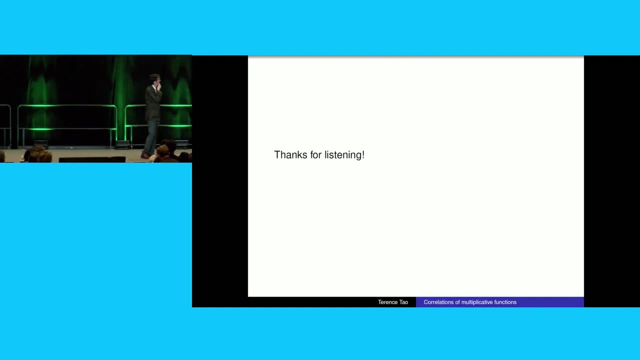 I mean maybe some of the audience may know offhand- I think there are. I mean you could just brute force search, but that's not the best way to find these large twin primes. I mean numbers that are kind of like Mersenne primes. 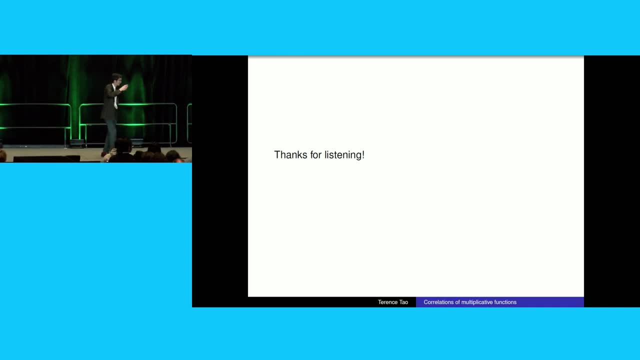 you know so not exactly Mersenne primes, but like powers of small numbers, plus or minus one times a constant. Those are fairly easy to check for being prime, And so I think the largest twin primes are kind of Mersenne type. 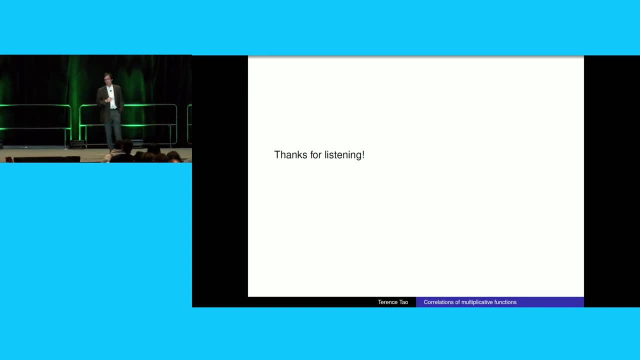 but I don't know roughly the number. Sure, okay, There is two. the number of two to the number of zeros is one in 12 million. Okay, So, yeah, there are some very large ones. yeah, Okay, time the constant and pass the mic on. 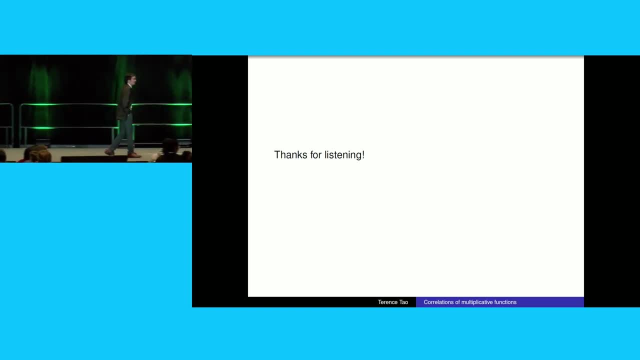 Okay, Hi, Yeah. so when switching from the, from the Mobius function to the Louisville function, do you lose a bit of the randomness? because the like the the pole at one half causes phenomena like the summatory function appearing to be negative. for the first billion terms or so. Is this something that comes up in practice in these results? Eventually it would, but if our error terms ever get below one of our root x, we would start noticing it. But you would need many things, including the Riemann hypothesis. 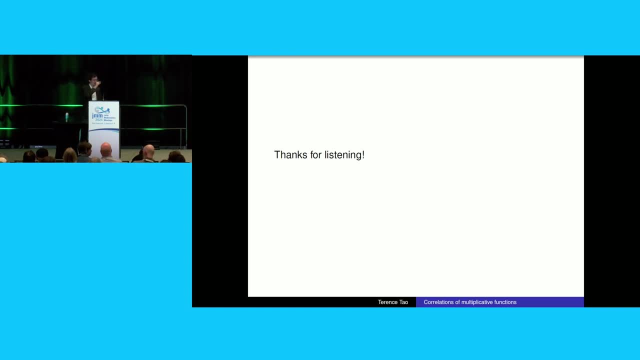 to even get that far, You know. so I gave this table of tiny improvements where we're shaving log, logs and logs and so forth. Yeah, so I. so that's coming from contributions from square numbers, And square numbers are really really sparse compared. 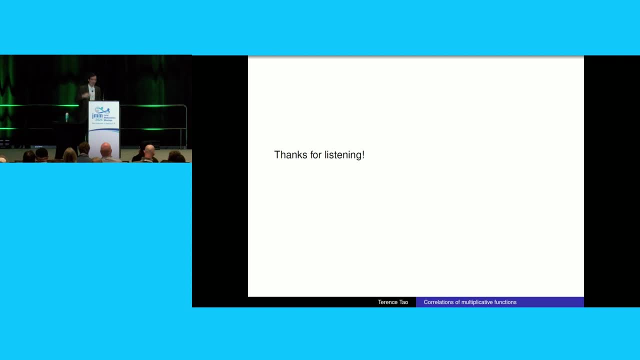 to prime numbers and all these other things That I mean. while it does make a small contribution, in the grand scheme of things it makes, it makes very little difference, At least for this part of number theory. There are other things like for Siegel, zeros and so forth. 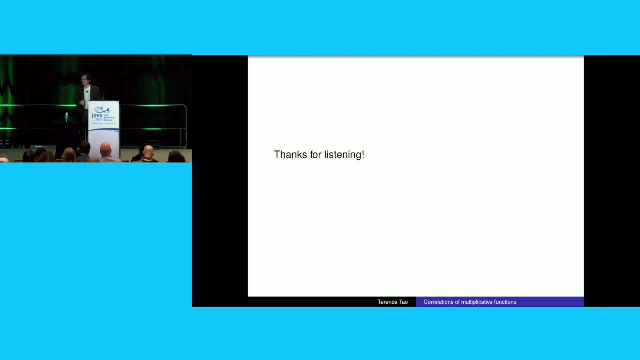 where these are important, But, yeah, not not for this area yet. Hello, It's a very nice talk. So it seems that many of the results depends on the conditions that the function, like the lower function, need to be multiplicative. 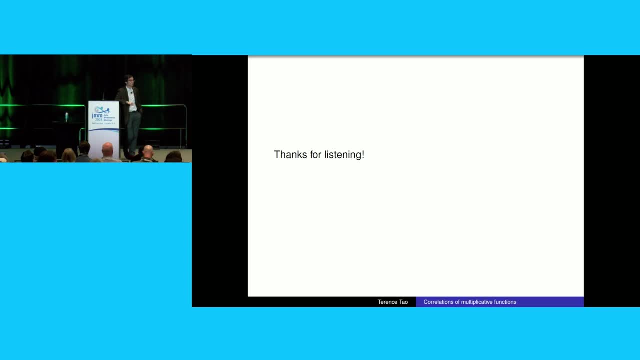 So have you think about it, if we can release this condition to some not complicative but maybe some weaker version of the That is. that is a great question actually. It's been proposed a couple of times whether how much of this theory extends to sort of weakly multiplicative. 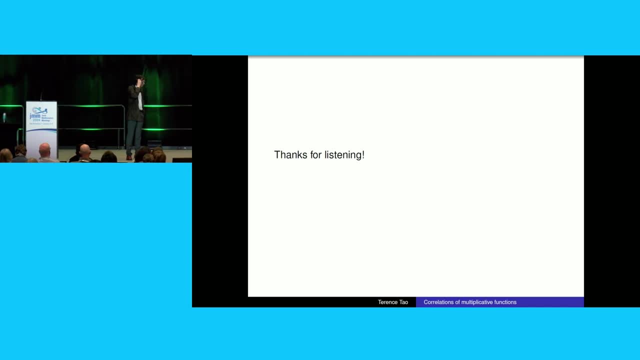 functions of some sort And there are some applications for this sort of thing. Like people consider things like smooth numbers or rough numbers, numbers that have all prime factors less than a certain threshold or something, And these are sets whose indicator function is kind of 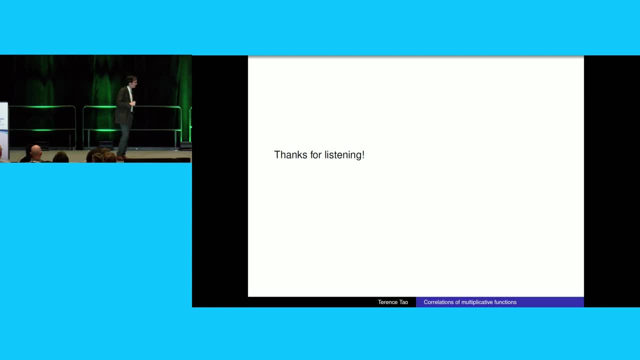 has approximate multiplicativity properties, but not completely multiplicative. So yeah, there are some extensions of this theory, but there's not really a canonical standard definition of what an almost multiplicative function is. Maybe there should be. Who should actually develop this theory? 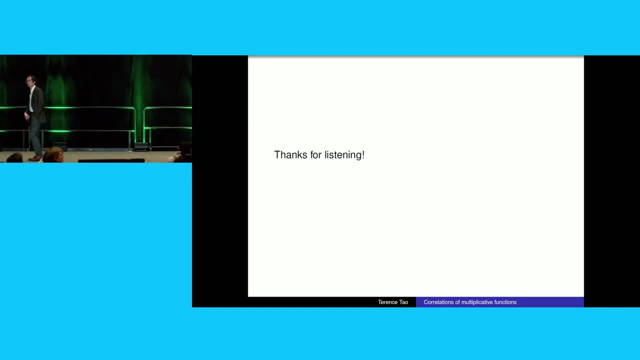 That's a good question. Thank you, Hello. So I know that in some places in mathematics sometimes the trick is to not study an object directly but to study a dual object, right? The first thing that comes to mind is perhaps the theory of functional analysis. 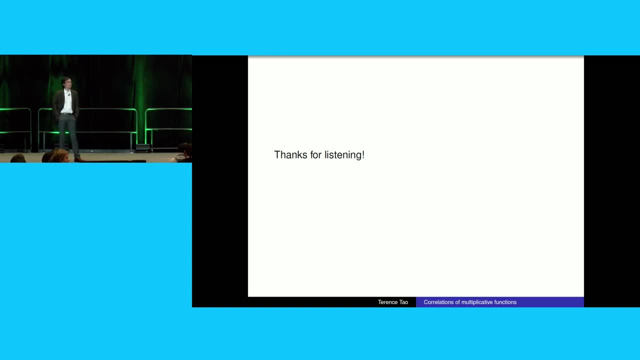 So I'm wondering: is there a good object already present, or can we come up with one? a good functional? Well, in multiplicative number theory there is. It's called the Riemann zeta function. Yeah, So yeah, we can take the Fourier dual of the primes. 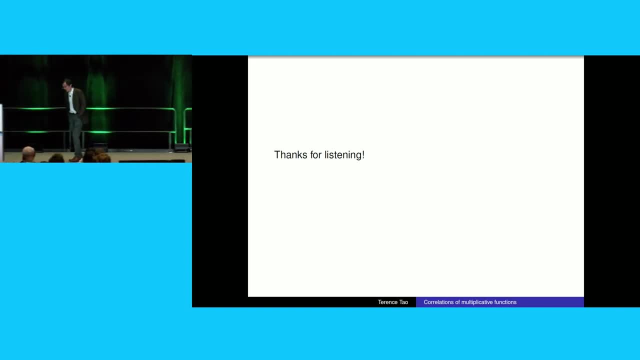 and that is basically the log derivative of the zeta function. Yeah, So if you have a purely multiplicative problem, then we kind of have a good theory. And also, if you also want to care about progressions, you also introduce characters. 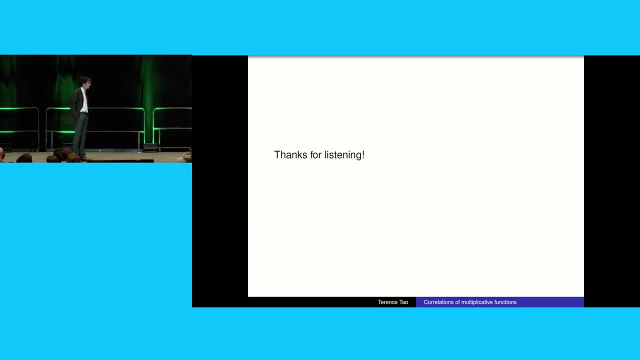 Yeah, Well, there's additive Fourier analysis, which we use a lot. Yeah, we don't have the sort of linearity that you kind of need to get a really good duality. There's not a category of a home and it's definitely not abelian. 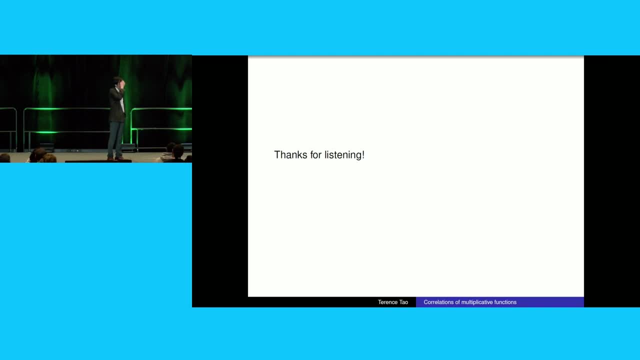 But in some sense I mean: well, we do study moments, a lot of these multiplicative functions, And studying the moments is again some kind of dual to the distribution itself And there are lots of theorems relating that, you know. 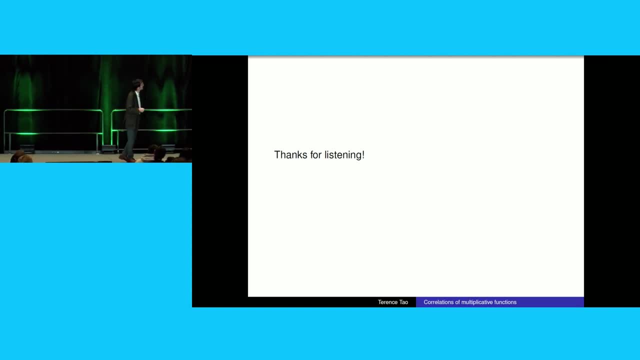 if the moments grow at a certain rate, then your distribution must do this, and so forth. Yeah, So there are various dual things you can do, and they're somewhat useful, But we don't have sort of a duality theory that sort of transforms the problem into. 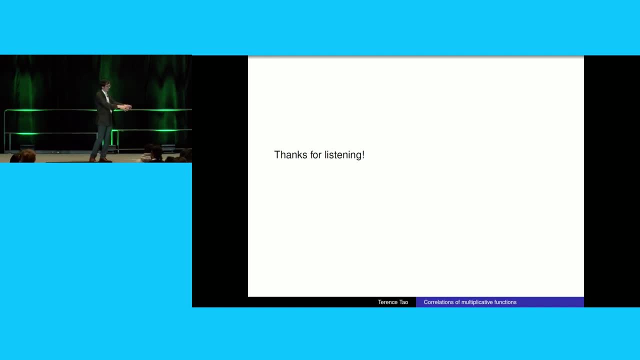 that lands you into a field where there's suddenly a huge bunch of new tools that you can use. Maybe there's one or two, and then you can go back and forth. But it's certainly a move you can do, but it's not a magic wand that solves the problem. 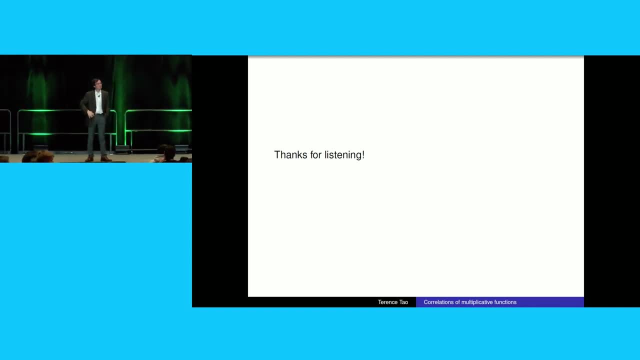 A follow-up question: If I have two integer sequences that I can apply multiplicative functions on and they agree after I've done this, can that be a technique or Well? so this, okay, I didn't briefly mention this single pretentious number theory. 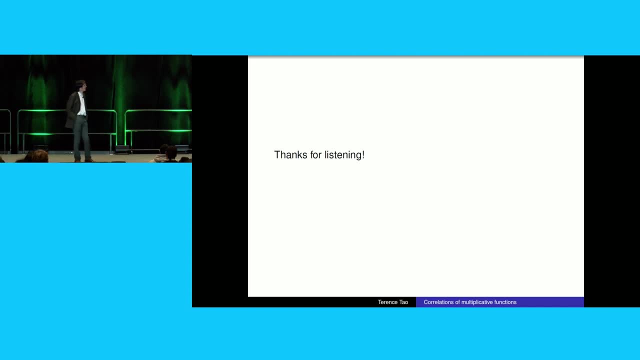 There is somehow this: there's a way to create a distance between two different functions, particularly multiplicative functions, by comparing what they do on primes in particular. And yeah, and if one sequence is another, sequence is twisted by a Dirichlet character. 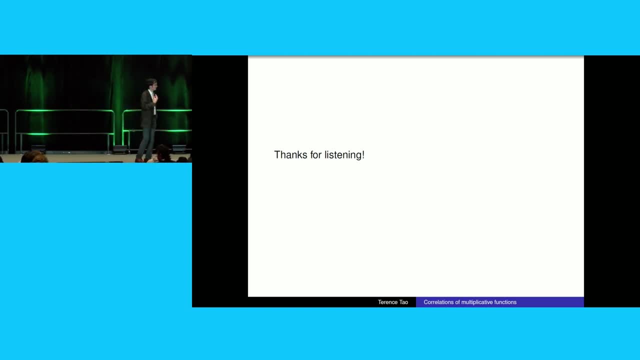 then they are related in various useful ways. Yeah, so there is some sort of geometry in the space of all sequences. that is very useful and at least certainly conceptually. yeah, so we, if two sequences are close in this metric. 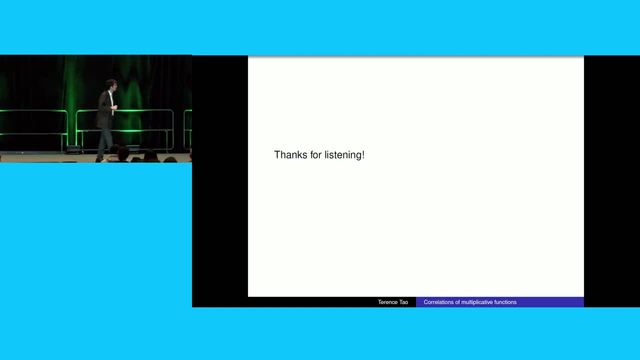 we see that one of them pretends to be the other, and it's a very useful conceptual notion, invented actually partly by my host here. But yeah, so I mean, yeah, it certainly it helps a lot to not just consider each sequence isolation. 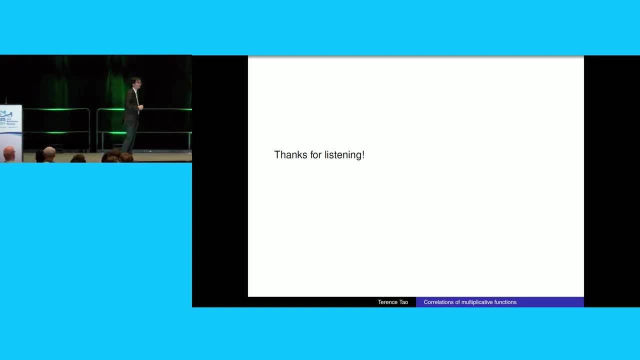 but how it relates to a lot of sister sequences. Thank you, Hi. thanks so much for your talk. Could you talk a bit more about the shortcomings of the sort of additive combinatorial- like density theorems- methods for tackling this specific problem? 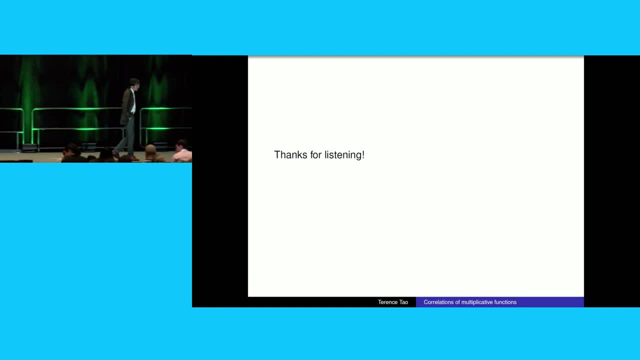 Well, so, for example, Zermatti's theorem is a great theorem if you want to count progressions. It says that that atomic progressions have a special property: They're somewhat indestructible, almost indestructible, Like if you have a set. 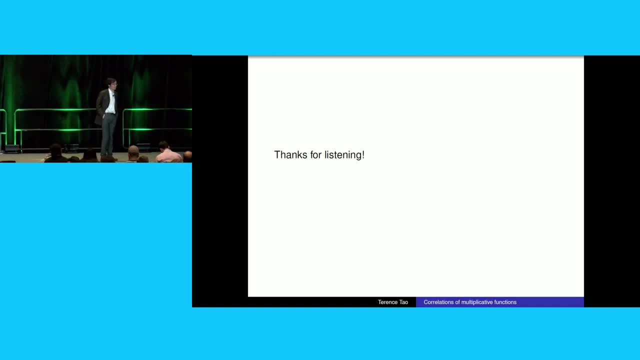 and you want to get rid of all the atomic progressions in the set, you need to basically delete almost the entire set. You have to make a set of zero density. That's the only way you can get rid of all the progressions. 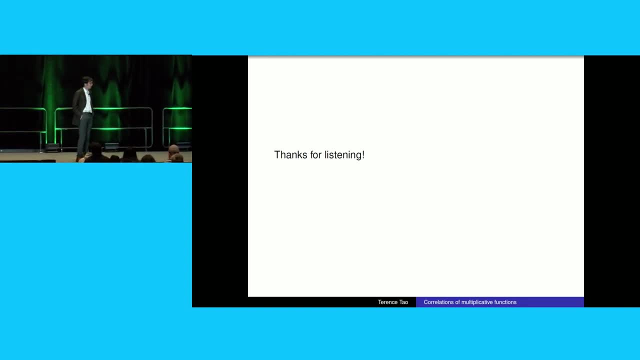 In contrast, if you have a set and you want to get rid of all the twins, you can do it fairly easily. You can basically identify all the twins and delete them. actually, it's the simplest thing to do, But there's also very dense sets. 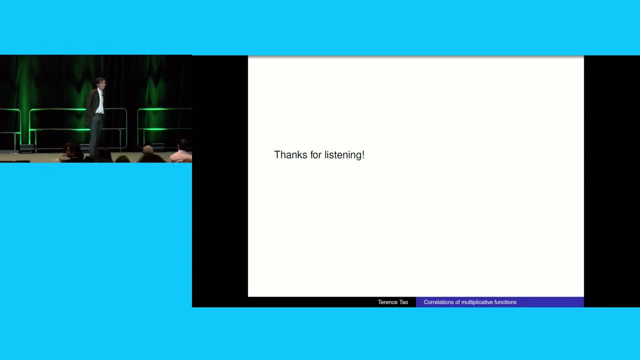 like the Mopsil 3, which have no twins. They have density one-third. So there are the, you know, standard asymptomatic combinatorics. things don't apply. There's a more technical reason, One thing that additive combinatorics has taught us. 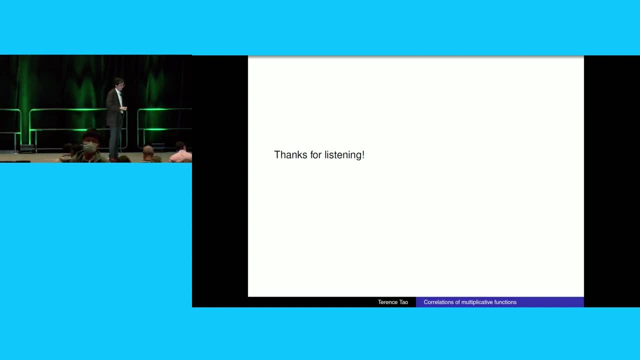 is that different patterns come with a number, called complexity. And so there's these complexity zero patterns that are very easy to count. complexity one: patterns which the circle method can handle. complexity two patterns. they need what's called quadratic Fourier analysis. 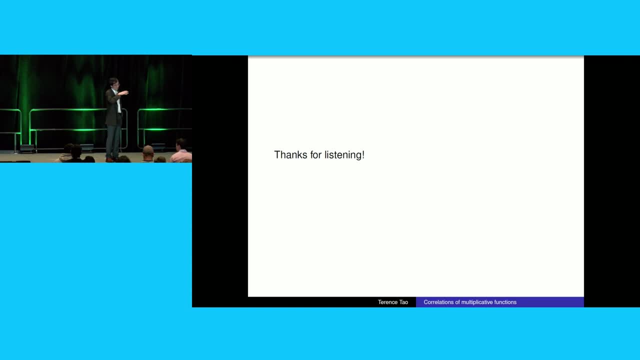 and so on and so forth. And asymptomatic progressions have this finite complexity and they can be handled by these additive combinatorics techniques, Twin primes- unfortunately twins have infinite complexity and none of our current technology can handle it. There are just too many ways. 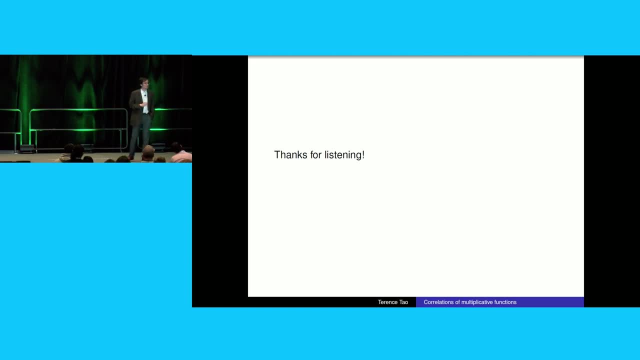 in which you can get rid of the twins for this type of strategy to be useful. Thank you. Thank you so much for your talk. At the beginning of your talk you were mentioning how the twin prime conjecture is, kind of this, somehow nebulous, but not nebulous thing. 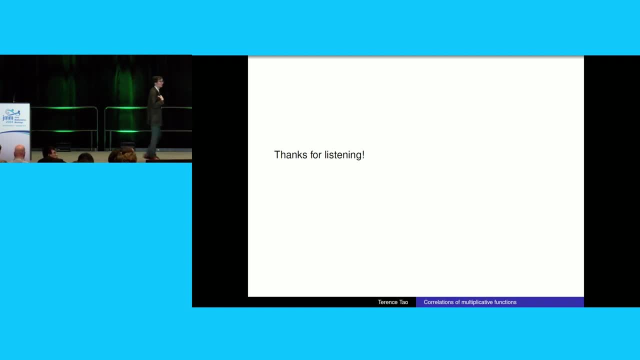 that we understand should be true, but a lot of the techniques that we have aren't quite good enough and sensitive enough to understand it. To me this was a bit reminiscent of results in other fields that also have other, I guess, big conjectures. 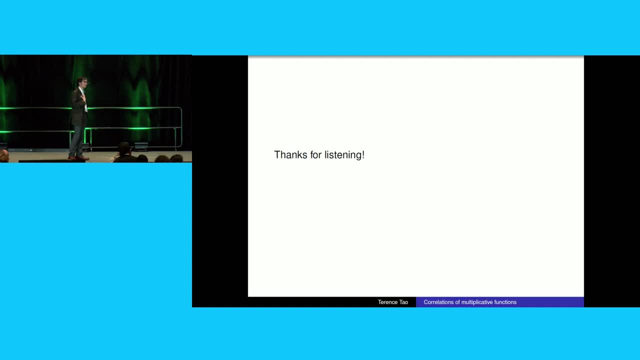 that we believe to be true but can't quite prove. For example, p not equals 10p, where we have things like the relativization barrier of how diagonalization could never work as a proof technique, because we need proof techniques that are sensitive to oracles. 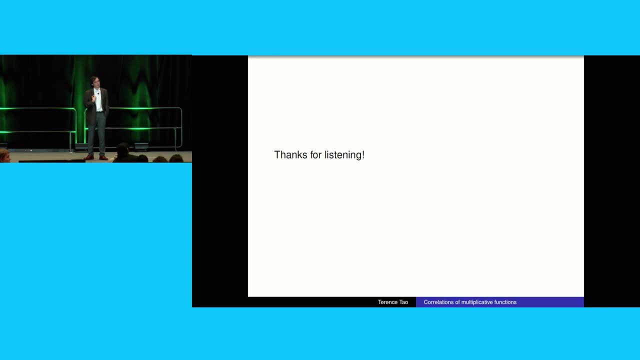 I guess I was curious if you had any sort of perspective that unified a bunch of these kind of big, unprovable, it seems, results by our current models. Our theory of barriers is nowhere near as advanced in number theory as it is in complexity theory. 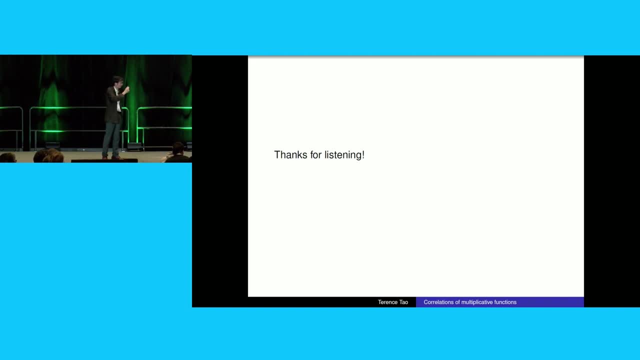 where we have this very precise notion of oracles, for example. I'll give you an example of a barrier which we've not been able to formalize. There are these hypothetical objects called Siegel zeros. These are zeros of not the zeta function. 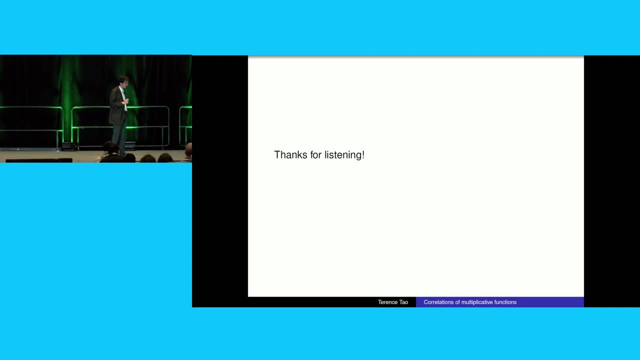 but a cousin called a Dirichlet L function that are very, very close to one. They shouldn't exist. The generalized human hypothesis is that they don't exist, But it's incredibly. people have tried for 50, 60 years to get rid of them. 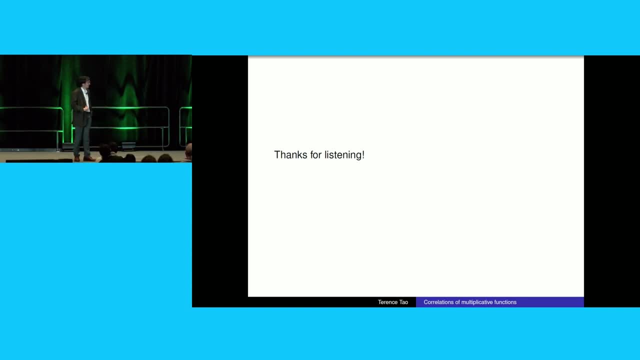 And they seem to be very stubbornly. they seem to want to exist. It's almost as if there's an alternate universe out there, which isn't our current universe, where Siegel zeros do exist, but this alternate universe is almost indistinguishable.